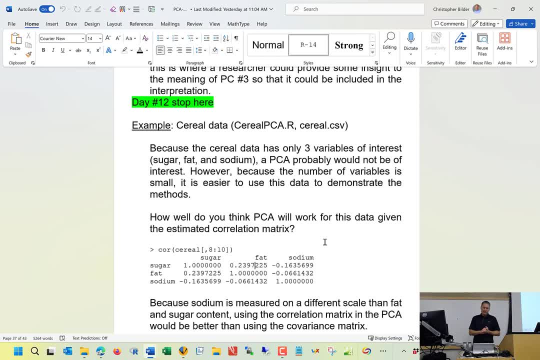 judgments, and we've seen that before. But since there's only three variables here, it help does help illustrate a few things more easily than if we had more variables. So first of all, let's take a look at the correlation matrix. So 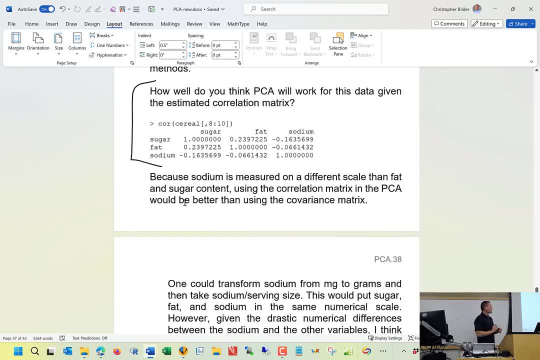 So, given this correlation matrix and what we know about principal component analysis- you know, don't worry about the fact there's only three variables- how well do you think principal component analysis will work in terms of its goals of, let's say, reducing? 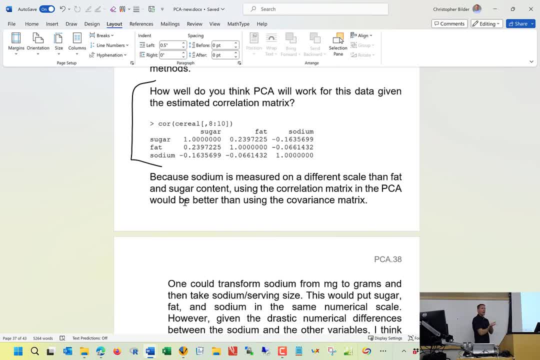 the dimension, or reducing the number of variables that you end up looking at. How well do you think principal component analysis will work, given what we see here with this correlation matrix? So you know, at the very beginning of the PCA section I said you know what PCA does. 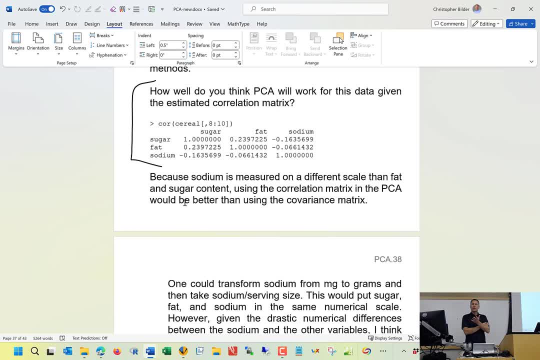 it takes a set of correlated variables and finds some new variables, called principal components, that are uncorrelated. What do you think about the levels of correlation that we see here, 11. Okay, Correlation is low, right, Yeah, And it doesn't work well. 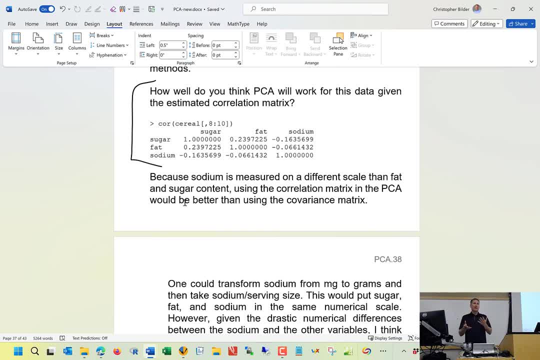 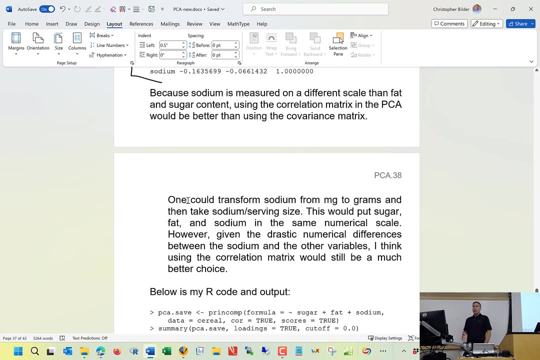 Yeah. So because of that principal component, analysis probably is not going to work well in terms of, let's say, reduce the number of variables, of these new variables that we look at in comparison to the original variables. Thank you. Now, also, in this particular setting, we will also want to use the correlation matrix. 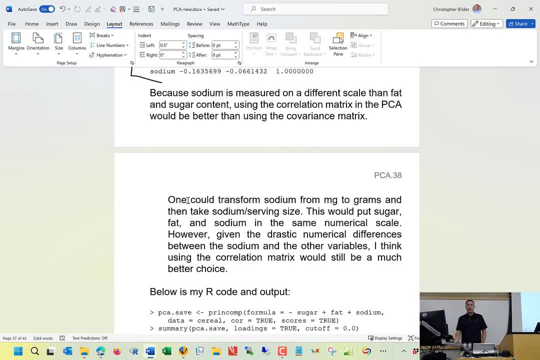 In other words, with our standardized variables, we will be using the covariates Covariance matrix, But people often will just refer to this as well. you're using the correlation matrix. Okay, We would want to use the correlation matrix here rather than using the covariates matrix. 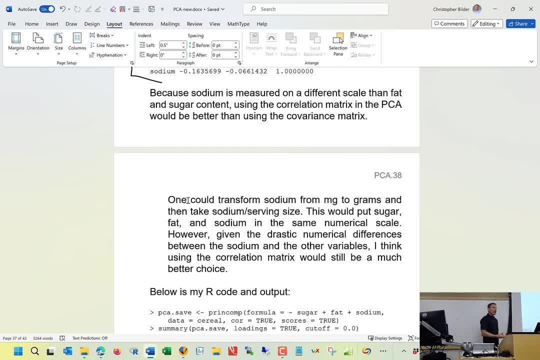 for the unstandardized variables, because we have variables that are measured in a different scale and also there's a vast amount of differences in the variability of these three variables. Okay, Okay, Now you might be wondering: well, couldn't we put these variables on the same numerical 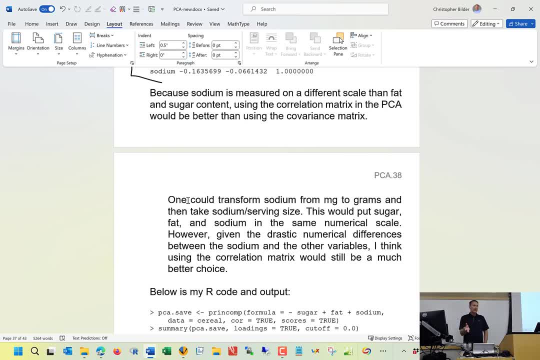 scale, because, after all you know, fat and sodium- I'm sorry, fat and sugar- are already, let's say, proportional grams per serving size and sodium is proportional milligrams per serving size. Well, can we just convert sodium to grams per serving size? 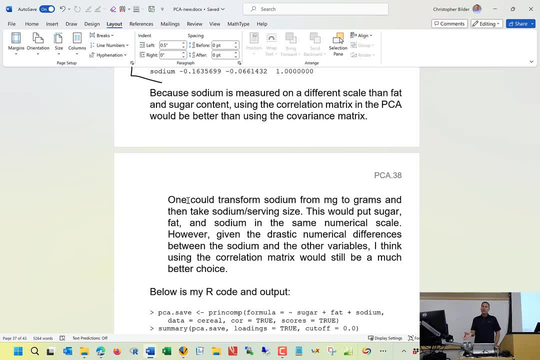 And, yes, you could do that, But you still will end up having a large difference in the variances of these three variables, even if they're measured on the same scale. Notice how this is different from what we saw with the goblet data. 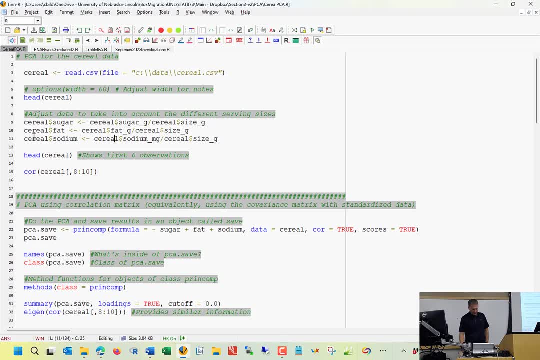 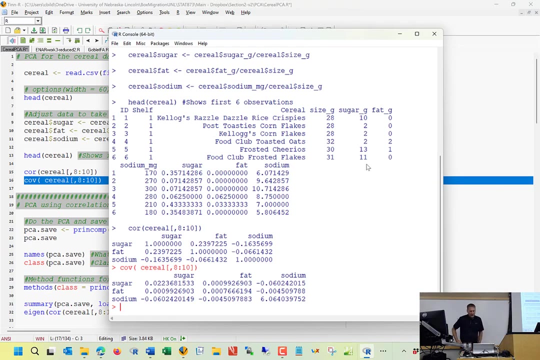 So I guess, just to actually illustrate this, Okay, Okay, Okay. So take a look at sugar versus fat. Look at the variances. We can see that the fat variance is much, much, much smaller than the variance for sugar. So that is evidence that indeed we want to use the correlation matrix. 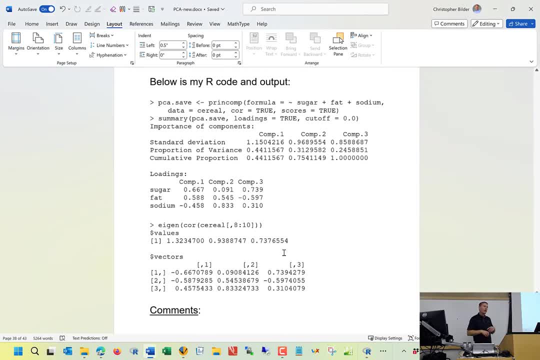 Okay. So to apply principal component analysis here again, I use the print comp function. I put my corresponding variables here. Notice how I say core equal, true, I do a summary of what's inside of my saved object. And so, for example, right here is the square root of land at star zero. 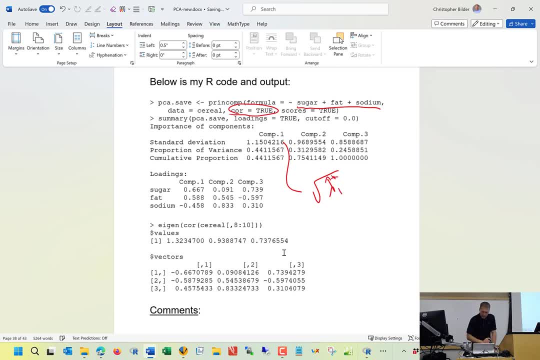 Okay, Okay Okay. That's the square root of land at star one. So my first principal component has a standard deviation of one point one five. Notice how the second principal component has a corresponding standard deviation less than one. In other words, lambda hat two. star is lambda. 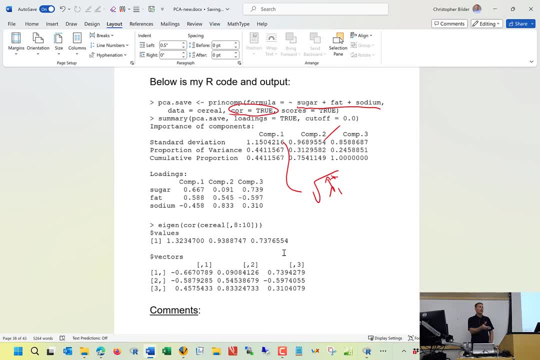 Okay, less than one. and remember, one of the criteria that we looked at for figuring out how many principal components that we would want to use would be to look at all of them that are above one. but if it's above one, we use it. if it's less, 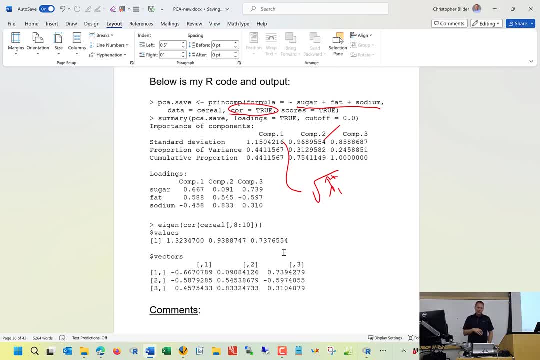 than one, we don't use that corresponding principal component. but again, I like to focus on proportion of variance so that first principal component has explains 44% of the total variability in your original variables. now, just three variables overall, each variable, when they're standardized, would explain 33%. 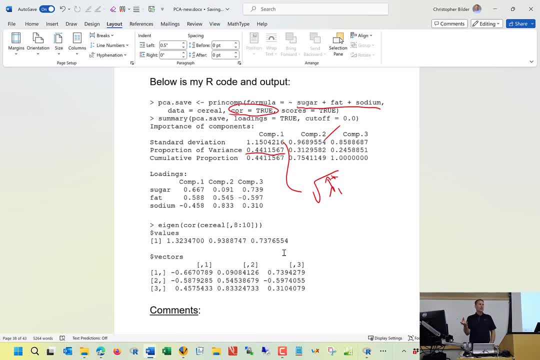 so you're not gaining much there if I look at- and I would never want to just simply use just one principal component. if I'm only explaining 44% of the information that's in my data, that's in my data, that's just not that much, so I go to my 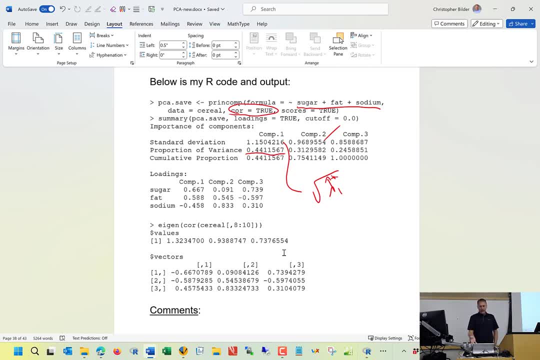 second principal component: okay, that's going to explain 31%. okay, notice how that's less than one-third. and so with that I'm explaining 75% of the variability, 75% of the information that's available in my data. it's not too bad. 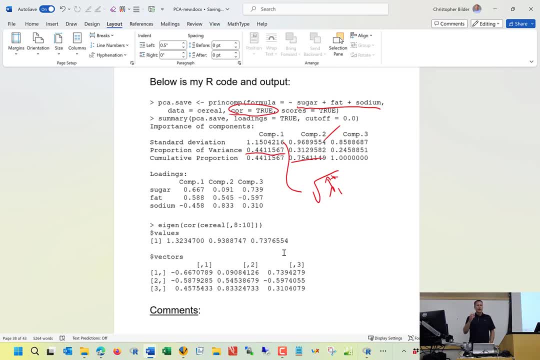 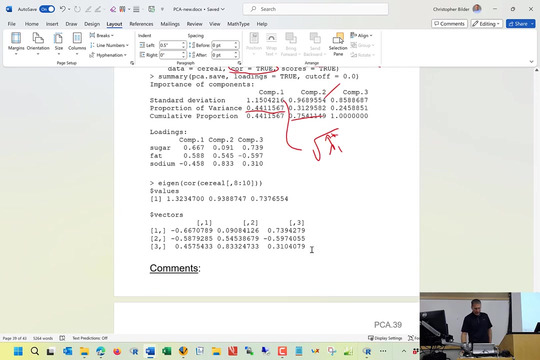 but then you'll think about this way I can use two principal components to explain 75% of the information that's in my data. when I only have three variables, why? why just use two? just just use all the original three. okay, here's something that's interesting. 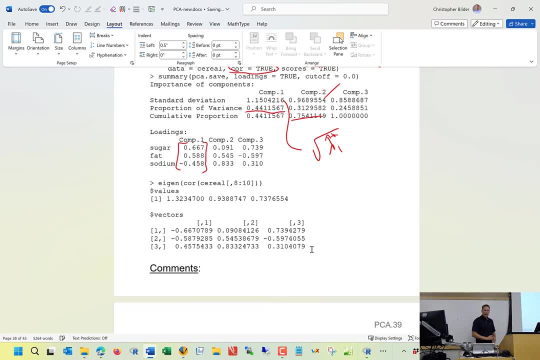 notice. here's something that's not too. Here's that first eigenvector, corresponding to the largest eigenvalue. How would you interpret, then, this first principal component? Just give me a simple interpretation. What do you think Let's see now? so it's almost like a steering contest. 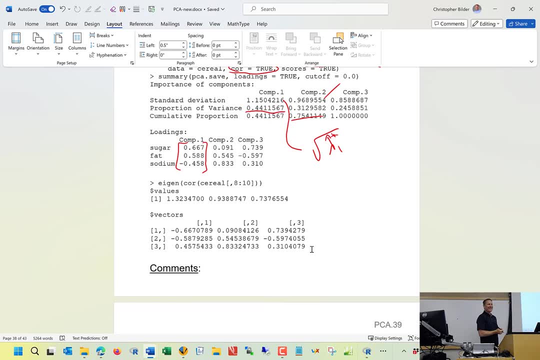 It seems that we have a large sugar on five. Let's see. Well, I wouldn't word it exactly that way. I would say it's a contrast between a combination of sugar and fat versus sodium. okay, So you know if I have a high fat, high sugar content cereal. 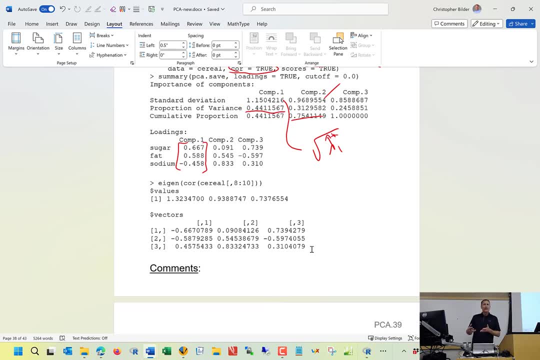 often the kinds that kids like I'm going to have a high first principal component value. Okay, Now I also use eigen with the correlation matrix, the eigen function- Notice, my eigenvector is a little bit different. Is this of concern? 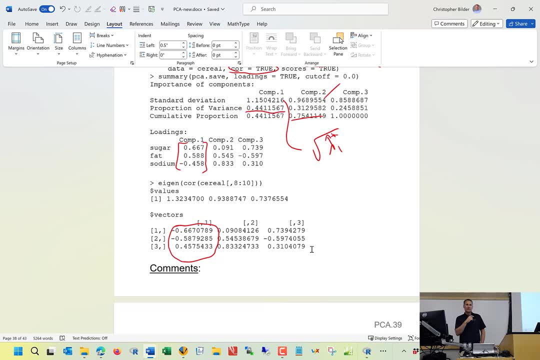 Did print comp do something wrong? Well, the answer is no. Why am I not? why is this not a concern? Well, think about it. What's that? I'm sorry, what? Well, think about it. What's the answer to that? 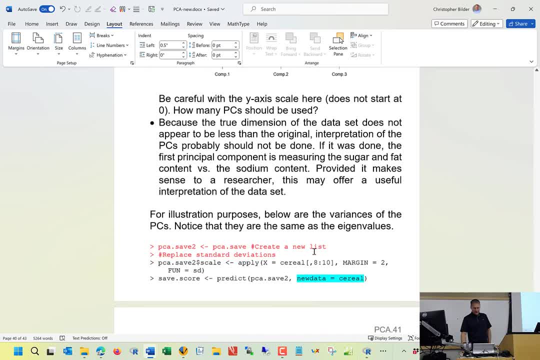 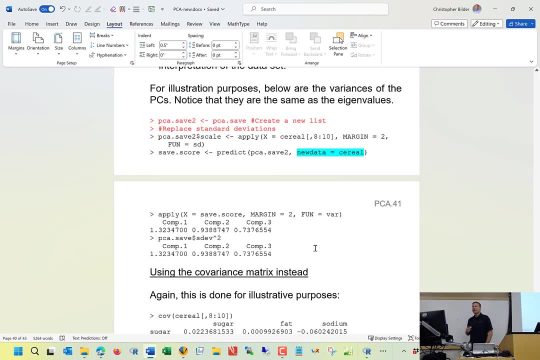 Okay, Now this next little part here is, I think, corresponds to maybe the very last problem of the project, and that is, I want to actually find the regular old sample variance of my principal component scores, And so one way to do that, 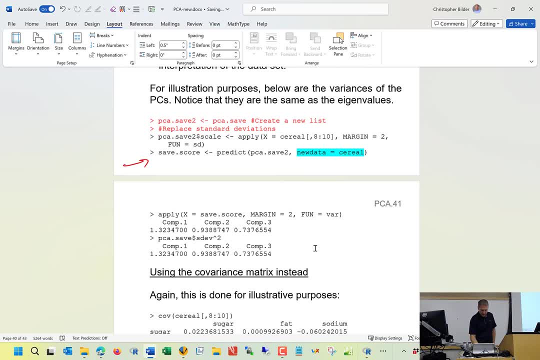 well, first of all I find the principal component scores, then I use the apply function where I'm going to apply to these principal component scores structure in columns, margin equal to. I'm going to apply a particular function to each column and the function I'm going to apply is var. so the sample variance. 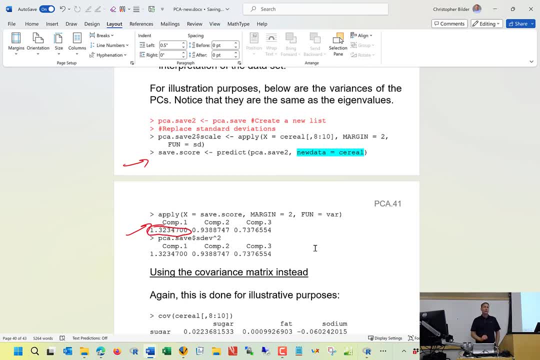 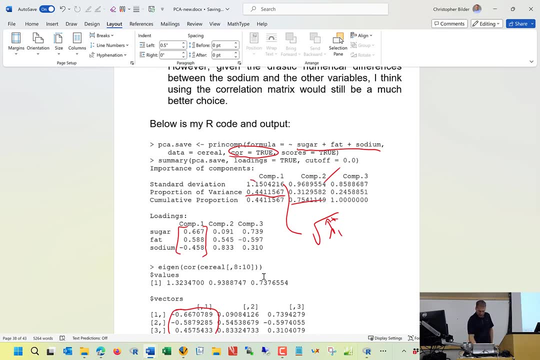 for all the principal component scores is one point three, two. and if I were to come up here to this right here, if I square that I get one point three, two. the purpose here is to illustrate that if I look at all the scores, sample variance is the same as what that first estimated eigenvalue would be. 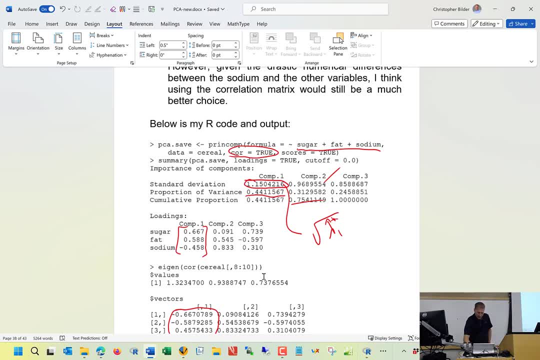 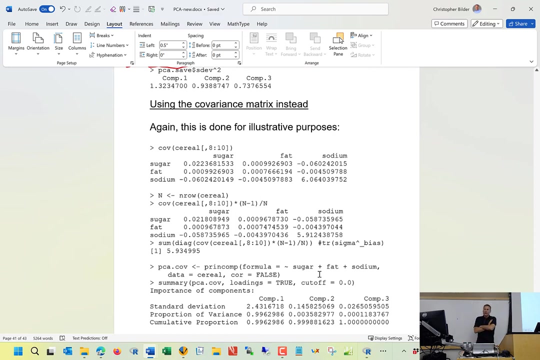 you. in terms of our notation, remember how we had var: one star is equal to lambda one star. that's what this is illustrating, but now we're doing it from the estimate perspective. well, what if, though? what? we did use the covariance matrix instead of the correlation matrix here, so again we're using the covariance matrix. 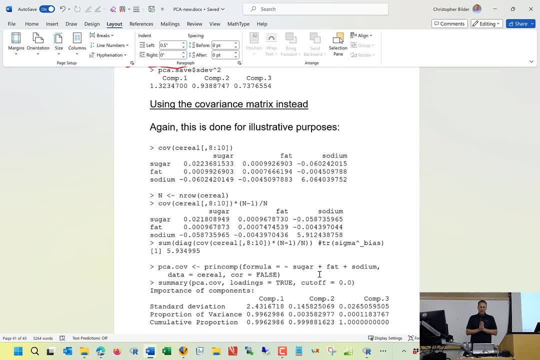 for our original variables. what, how bad would it be? so here's that covariance matrix again. I already illustrated this big difference that we see here. but then also compared to sodium. look at that, that sodium is much, much bigger. so what if I now use this covariance matrix with print comp? so I would say: or equal, 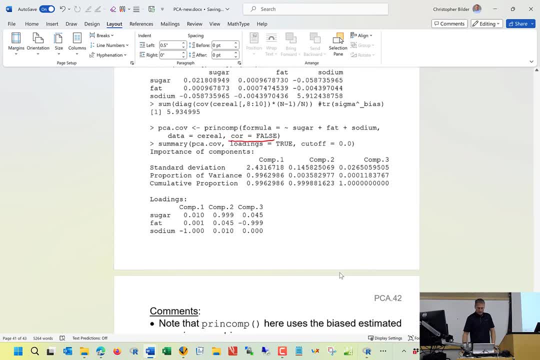 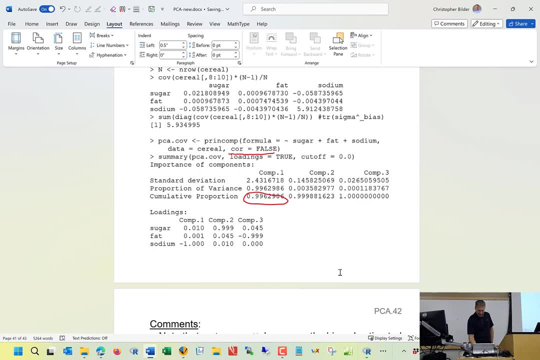 false. now this is what I get. the first principal component explains ninety nine point six percent of the total variability of my data set. but what's going on here, why? why is this so much higher? take a look at that first eigenvector. take a look at that first eigenvector. 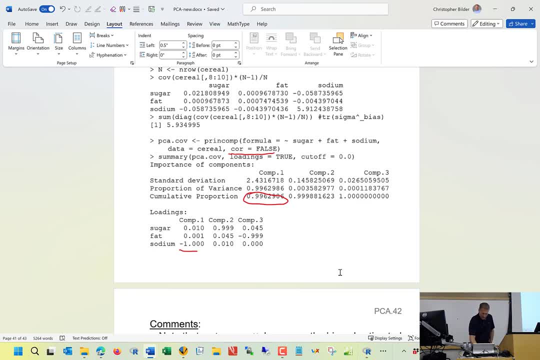 sodium has a negative one. there, sugar and fat are essentially about zero. so what is this first eigenvector? I'm sorry, what is this first principal component representing essentially just sodium? why did this happen? well, this corresponds to something that we actually talked about in our last class principal component. 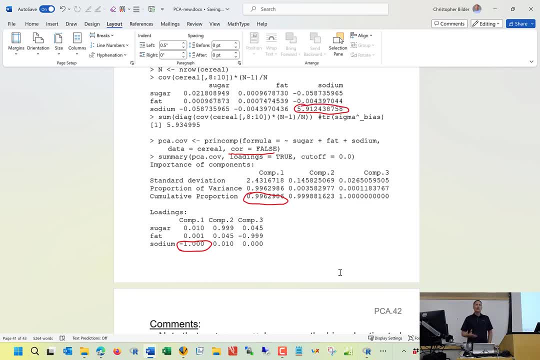 analysis notices that that variance for sodium is so high. and so if I look at my total variance and if I want to explain as much of the total variants as possible with this linear combination of my original variables, it would make sense that let's just put a whole bunch of weight on sodium. 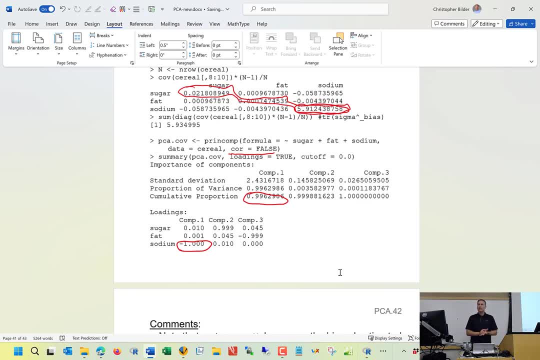 and wallah. I've explained on ninety point six percent of my total variation. take a look at the second principal component. It's essentially just representing sugar. Why? Look at how much bigger the sugar variance is compared to the fat. The third principal component is essentially just only fat itself. 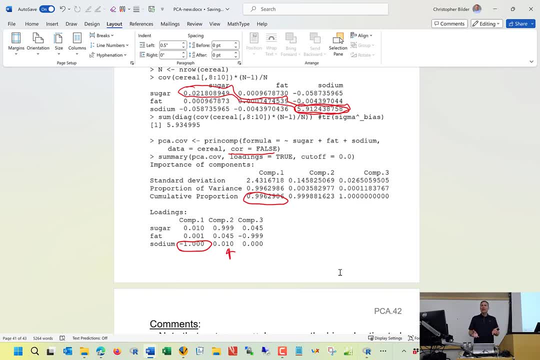 And so is this principal component analysis worthwhile? No, because, essentially, you're just getting back the original variables themselves. This then, I guess, puts a data example to what I had talked about before, about what happens if you do have a lot of different variances amongst your data. 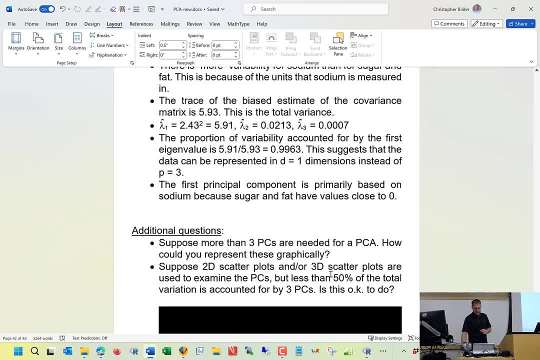 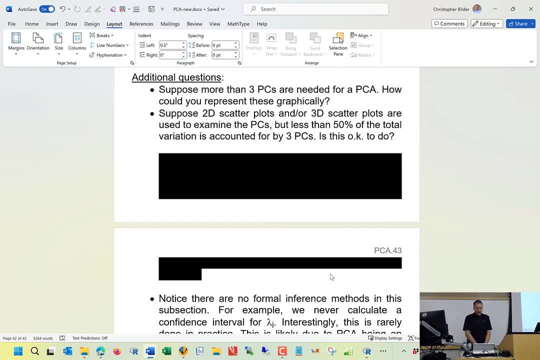 Any questions about that? Okay, some additional questions, and then we'll be done with this section or set of notes. Suppose more than three PCs are needed for a PCA. How would you represent these graphically? We actually already talked about that. 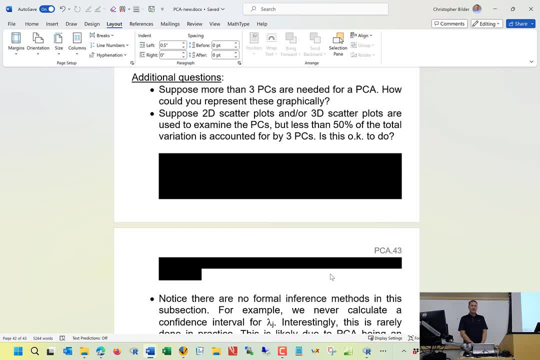 Does anyone remember what the answer is? So let's say I want to. let's say I need five principal components to get, let's say, 90% of the total variability in my data. How would I represent them graphically? I can't do a 3D scatter plot. 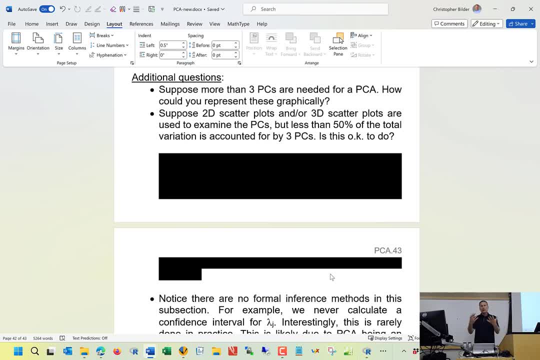 Coordinate plot. Yeah, the parallel coordinate plot. If you don't have too many variables- I'm sorry, too many observations- you could use a star spot as well. Suppose 2D scatter plots in or 3D scatter plots are used to examine principal components. 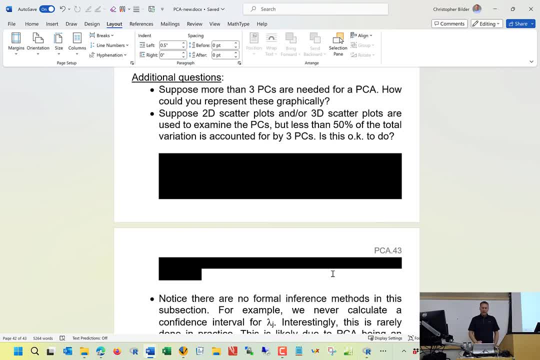 The scores, But less than 50% of the total variation is accounted for by these three PCs. Is this okay to do? What do you think We might have talked about this also a little bit earlier? Would you be comfortable doing? you know, let's say, two principal components explain 45% of the total variability. 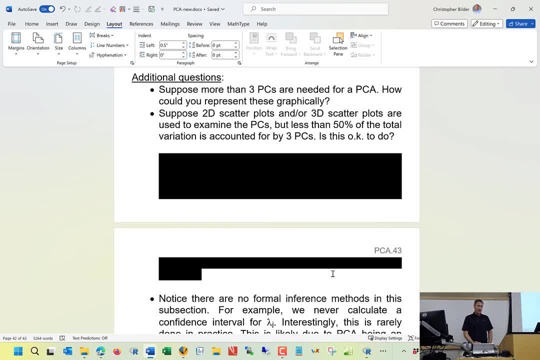 that total information that's in your data, And you did a two-dimensional scatter plot of them. Would that be okay? I think so. Why? I'd say it's kind of Well. I mean, this explains some information about your data, right. 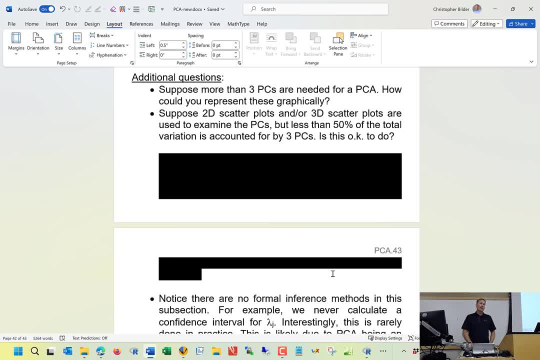 45%, But you could be missing a lot too. right, So it's common to still see people do that, You know, to do the scatter plot, But you really need to say: wait a second, I could be missing some information. 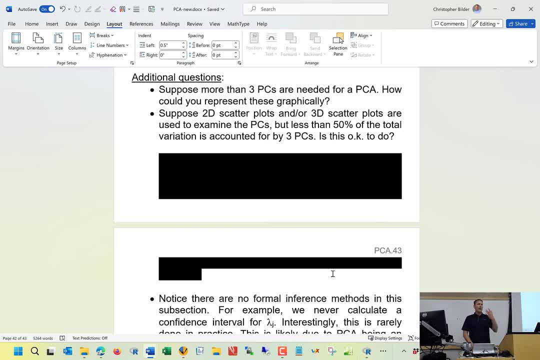 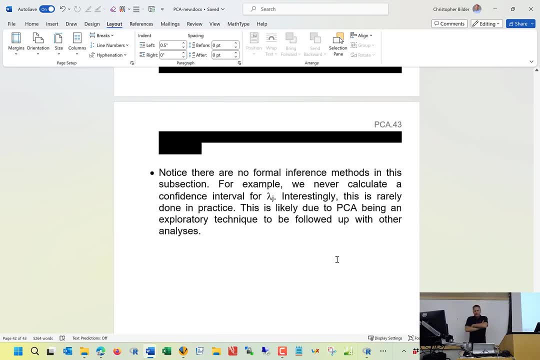 Okay, And still follow it up with like a parallel coordinates plot, Okay. And then, lastly, here there are no formal inference methods in this part of the notes, So I'm not doing confidence intervals, I'm not doing hypothesis tests. 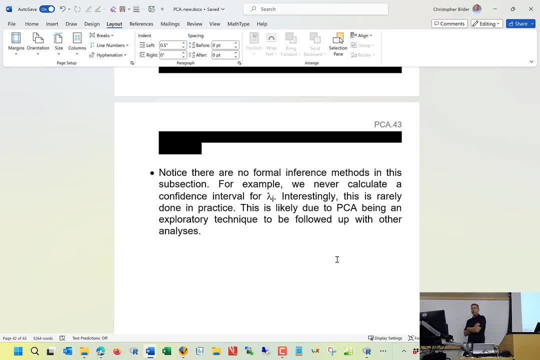 And you know you might think, okay, well, you could do it for the Lambdas, Maybe that might help you make a judgment of: okay, well, do I need two principal components, Do I need three? But this is rarely done in practice to use inference in principal component analysis. 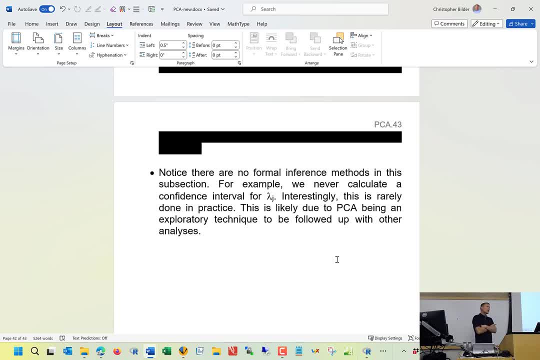 And the reason is is because principal component analysis it's often thought of as more of like an exploratory technique. Okay, To get an initial examination of your data, for example, Rather than this is the final end analysis that you're going to be doing. 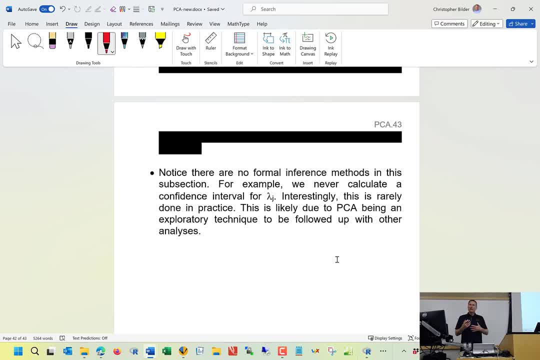 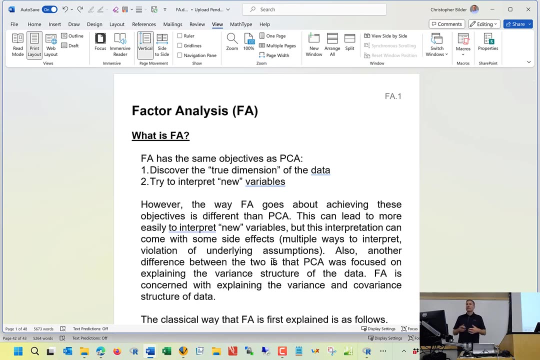 And so that's why you typically don't see people use inference methods with PCA. Okay, Any questions before we move on? Okay, so next we're going to talk about factor analysis, Or I'll just often abbreviate with FA, And there's a lot of similarities with principal component analysis. 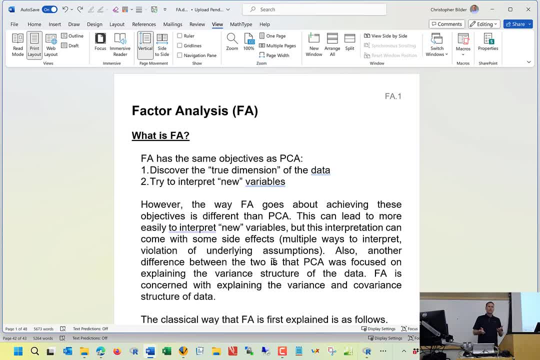 In terms of the overall goal is to, let's say, look at your data in a smaller dimension Or find the true dimension of your data. So, again, if you start off with ten variables, Maybe I could find some combination of these variables. 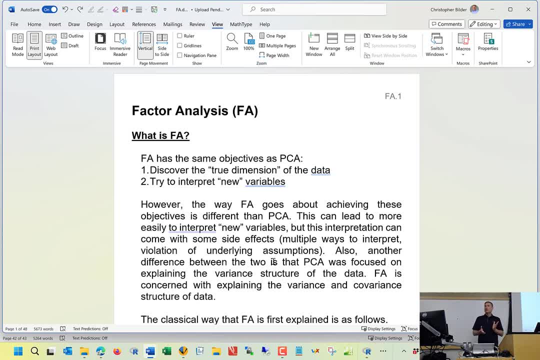 Such that maybe only two are really needed So that I can still understand what my data is giving me In terms of the information that's available. So that's same as principal component analysis. Also, these new variables that you form, You would like to be able to interpret them. 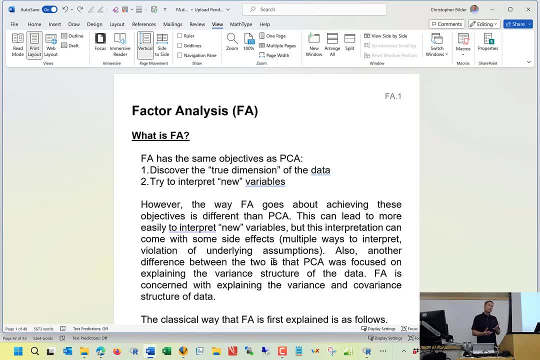 Now one From one perspective. An advantage that FA has over PCA Is that you can potentially have more luck with getting a good interpretation of these new variables. However, Getting this Maybe easier interpretation has some side effects. Okay, Now I have to admit that. 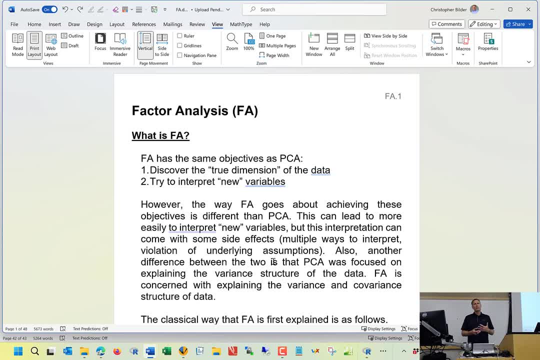 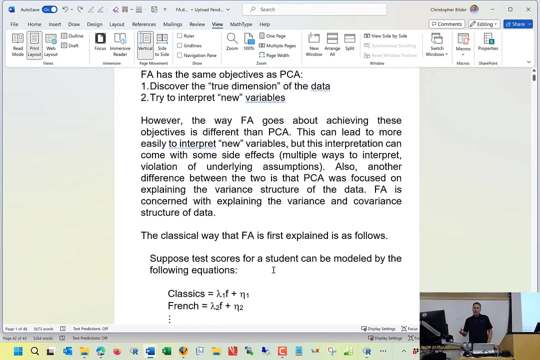 You know I will use principal component analysis. I will rarely ever use factor analysis, But factor analysis is widely used, Especially in the social sciences. Now the way that factor analysis Obtains these new variables is different And you'll see as we come along. 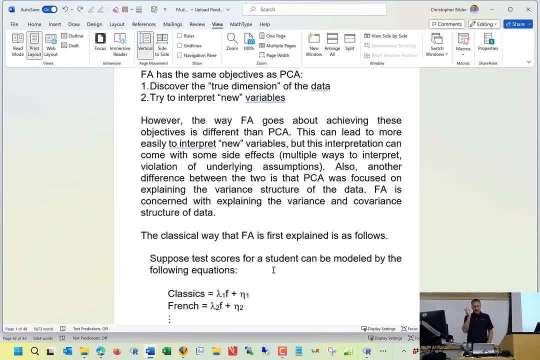 You'll see more about that as we go along. But You know, With principal component analysis We were very interested in the variances Of the original variables. In fact we said, Okay, You know If I explain 80% of the total variability in my data. 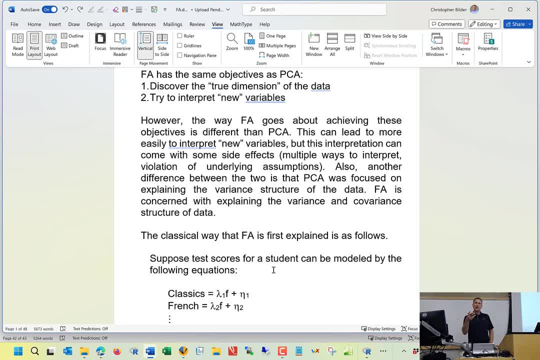 That's good. I'm explaining 80% of the information in my data, But You would also think about Well, Information though, itself Shouldn't just only be based upon variances Of the original variables. How about the co-variances as well? 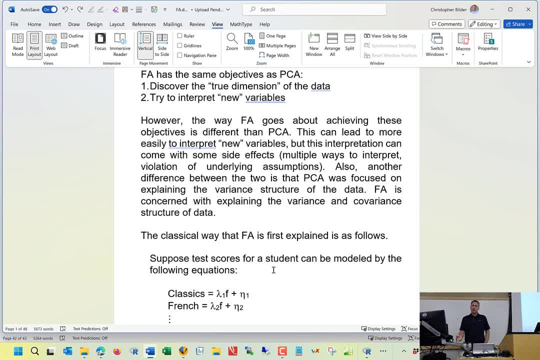 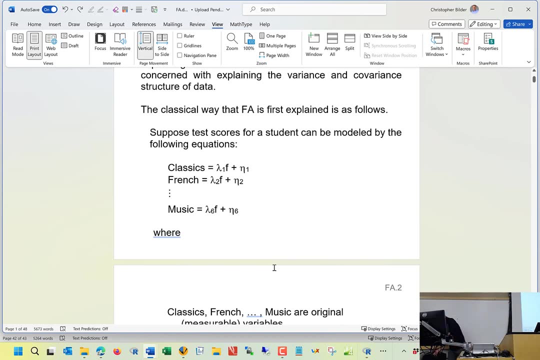 And that's what factor analysis Tries to do. Both the variances and the co-variances Try to explain those. So here's the classical way that Factor analysis Is usually introduced In a multivariate course. It actually goes back to: 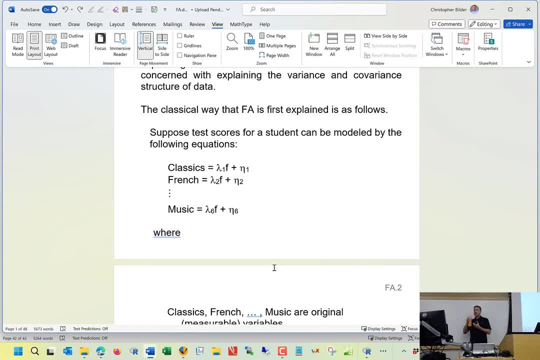 Some of the original Formulations of the ideas behind factor analysis. I think the very first paper On factor analysis basically used this. It's kind of a: You know There's a, There's a long history with this And so. 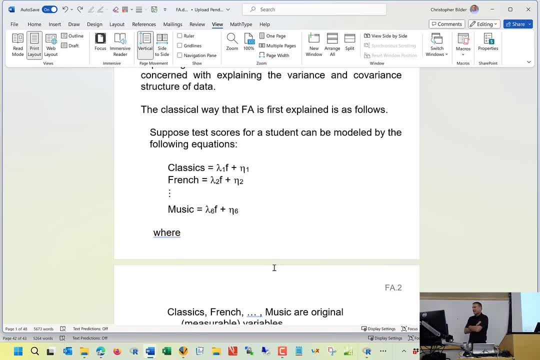 So the example is, I guess, has some old concepts to it, And here's, Here's the classic explanation. You know, Suppose we have test scores For a student And they're taking classes Like The classics French Music. 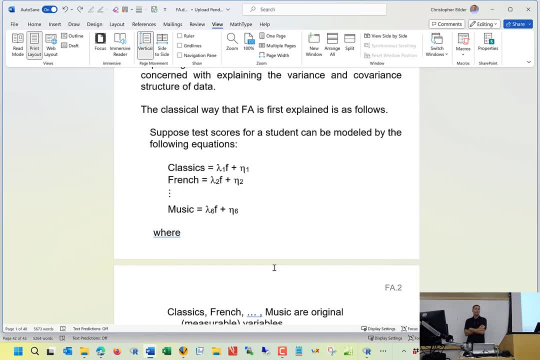 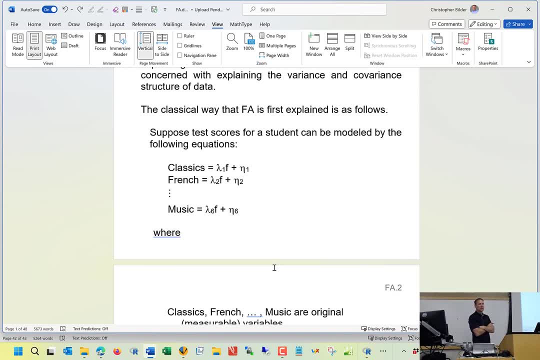 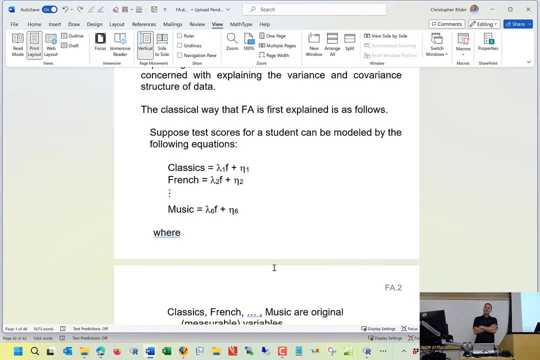 And you might think that You know Maybe. How well A student does Is dependent upon Two main things. One, overall intelligence level. if you could somehow measure it, Yes, maybe some student who has a really good overall- again this is the example- has a really 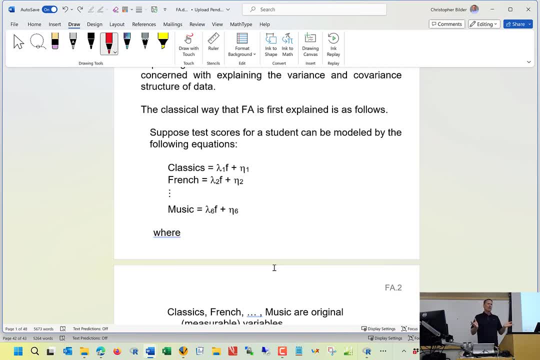 good overall intelligence level. well, you might expect their, their test scores overall, to be higher than maybe the student doesn't. But also another, let's say, factor that might come into play with these test scores is that maybe a student really, really, really likes French and maybe doesn't like music at all, And so 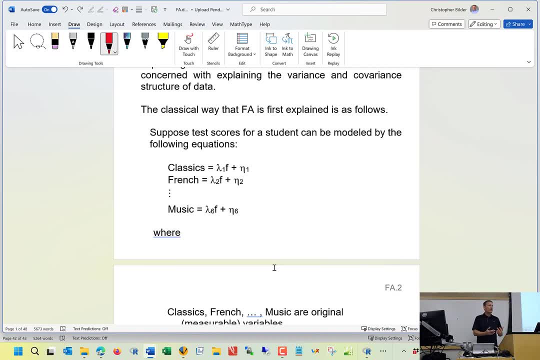 there might be some subject dependent factors that could lead to higher or lower scores, And the way that we can put this in a, let's say, a mathematical context, then, is what's shown here. So maybe overall intelligence level, let's call that F. This is something that's. actually unmeasurable. I don't have you know. sure, you could take like a IQ test or something like that, but that's not getting at it directly, your overall intelligence, Unlike you know. let's say, if you measure your height, well you know, it's only for me like six foot two. Okay, that is my measurement, but you can't. 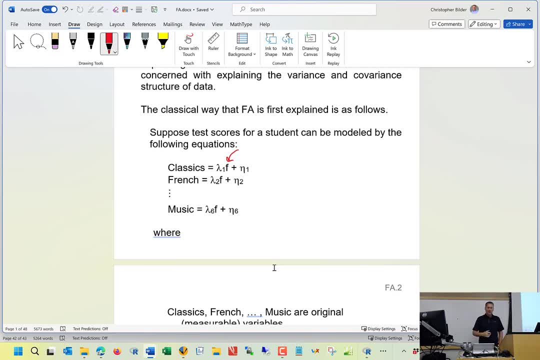 measure my overall intelligence And so, common to each of these class test scores, we have this overall intelligence, Where how much weight overall intelligence matters, corresponds to these lambdas. Think of it like a regression model. Like you have a beta, You know how much weight does a lambda have and how much weight does a 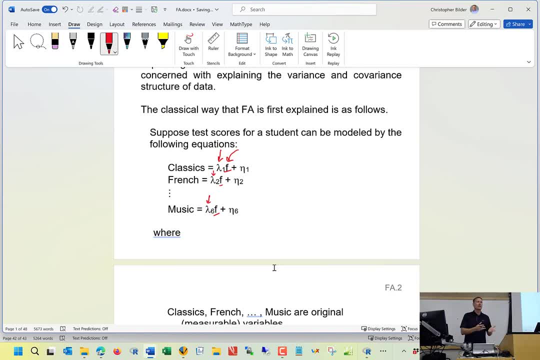 beta have. So the weight you put on that beta corresponds to how, let's say, x affects the response. So if let's say lambda one was zero, that means overall intelligence doesn't have play a role at all into the classics test score. If 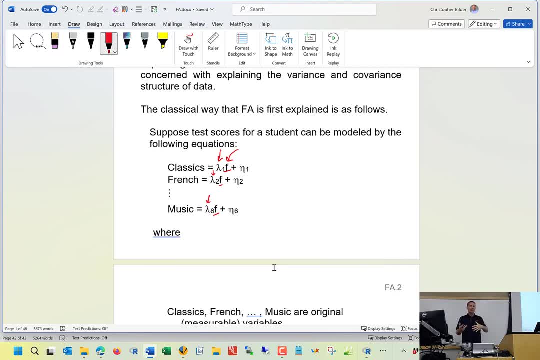 lambda one was positive, then it has a positive effect. If lambda one was negative, it would have a negative effect. Okay, since this F is in each of these equations, F is referred to as a negative common factor. It's a factor that goes into what the overall test score would be for each of these grades. This lambda is called a factor loading, So notice we're using it. we've seen that loading term before in the PCA section And it has kind of a similar meaning here in terms of it's like a weight. 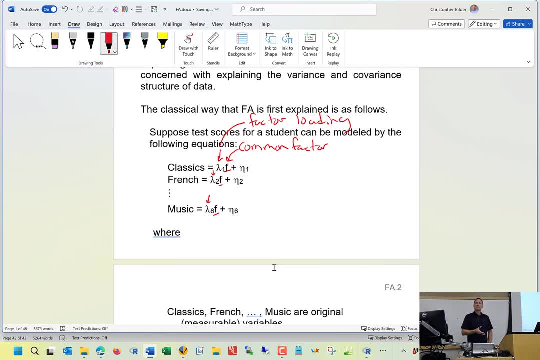 It's a weight on the common factor. And then, lastly, we have these other. we have these other things that are subject, class specific, So they are called specific factors. Notice how I'm using the S: specific factors. So there are six specific factors. 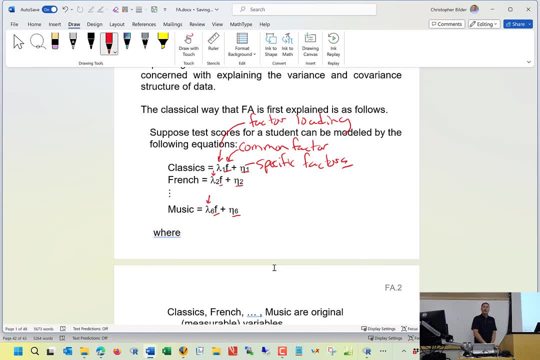 And that's actually unmeasurable as well. Think like with a regression model where you know you have some independent variables, your axis, At the very end of your regression model, what do you have? You have that error term. You have what's often referred to as epsilon. That's unmeasurable as well, And the goal there is to, let's say, with that epsilon, to look at all the other information that you're not measuring. 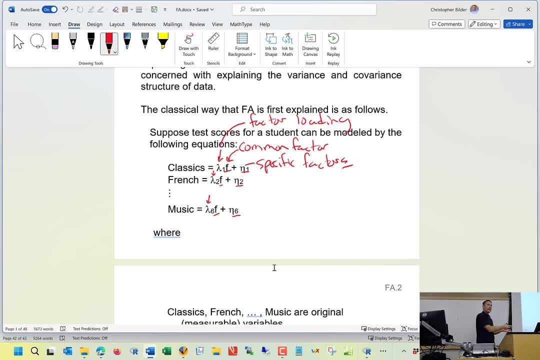 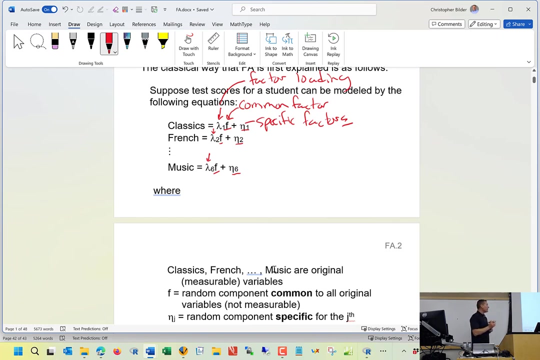 In terms of your x's And that's going to give you your y in the end, And this kind of has a similar meaning. So there are some here, some factors that are specific for a particular course. Okay, And so if you somehow know lambda one, you know f and you know that is the Greek letter eta. 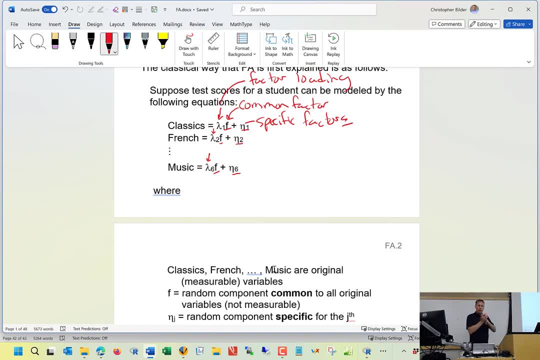 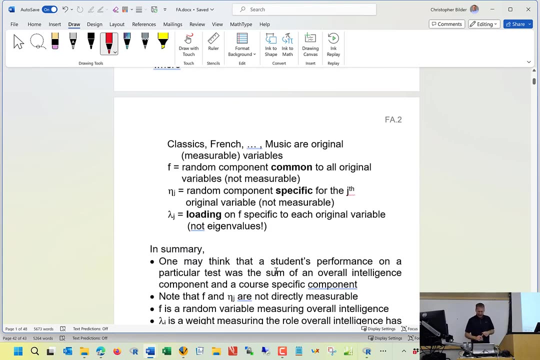 So if you know lambda one, you know f, f, eta one, You get that person's classics test score. If you know lambda two, f and eta two, you get the corresponding French test score. Okay, So let's see if I can make sure I talked about all this here. 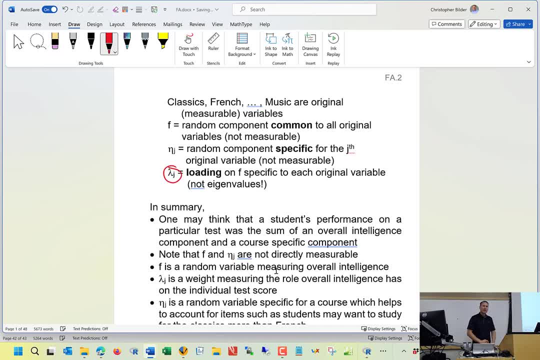 So be careful here. You know we're using this lambda here. Just be careful. It's not an eigenvalue. This is just a common notation that people use. That's why I ended up using it. So, even though we've used lambda before to represent an eigenvalue, it's not here. 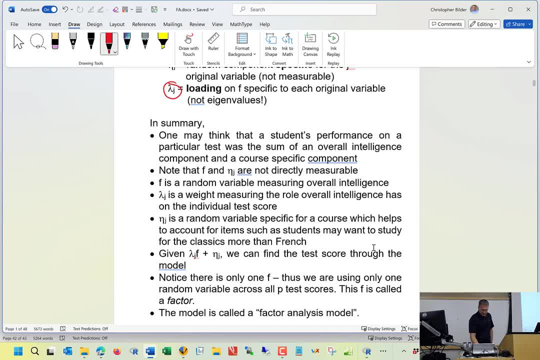 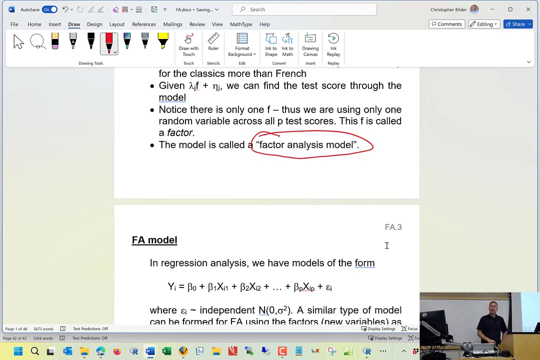 Okay, Let's see here. So f, our common factor, is a random variable. Lambda j is a weight on this f. We will want to estimate this lambda. Eta sub j is a random variable as well. Okay, So what I've just presented to you is what's called a factor analysis model. 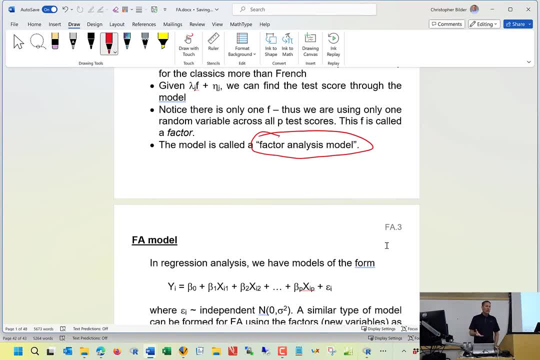 You see some similarities to what we've seen, what you see for a regression model, You know. but there are differences as well, Because, notice, we have an equation, We have multiple equations, Not just one equation, But we have multiple equations for the regression model. 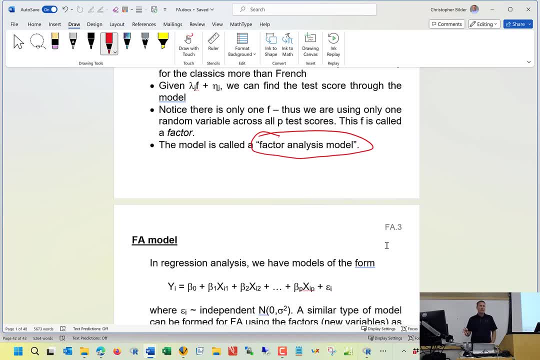 Now, overall, let me warn you, in this whole set of notes there's a lot of terminology. You know, if I was the one who was developing factor analysis, I wouldn't introduce all this, I wouldn't do all this terminology. 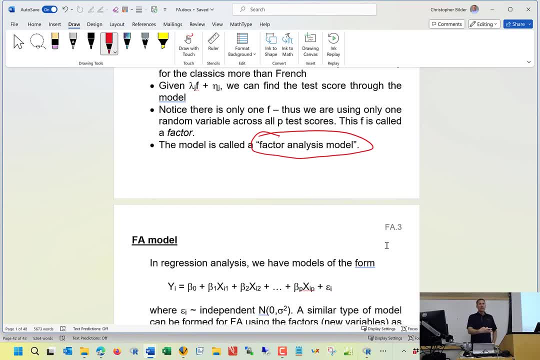 But I'm going to give you all this terminology because you know, especially if you use this outside this class, you have to be ready with understanding. okay, this means this. this means that: Oh, this has two different words that represent exactly the same thing. 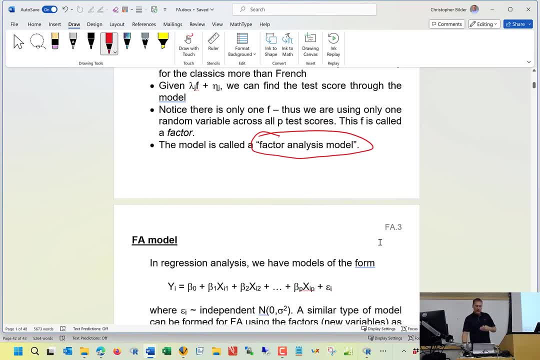 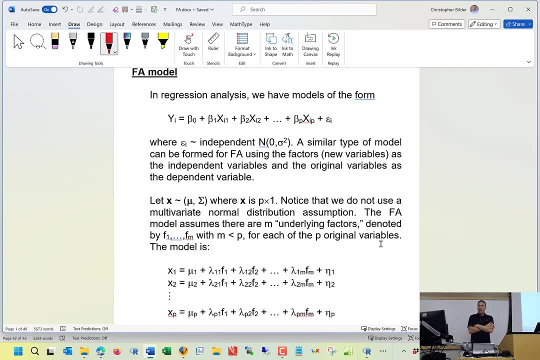 So that's why I'm going to give this to you. So just realize there's going to be a lot of terminology. Obviously, we just already introduced some terminology. There's going to be a lot of terminology And I think probably in all the notes that we have in this course, this is going to take me the longest: to go through some introductory stuff before I get to an actual data example. 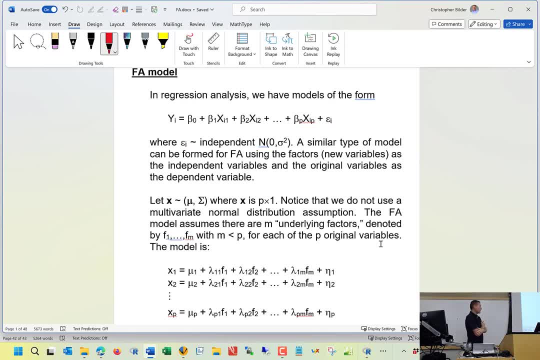 Just be patient. We will get to data examples coming up. So let's do this. let's talk about this relationship between regression analysis and what a factor analysis model is a little bit more So with this regression model. here's just kind of a review. You know we have this y, that's our response variable. 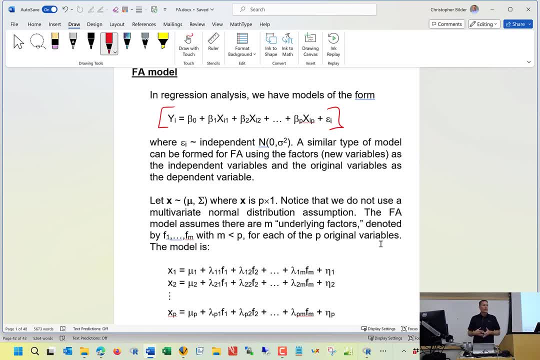 X's are our independent variables or explanatory variables. The betas weight each of the x's to give us some information about how x affects What. At the very end of the equation we have an epsilon. this epsilon represents our random error term and basically just this, basically just represents everything else that 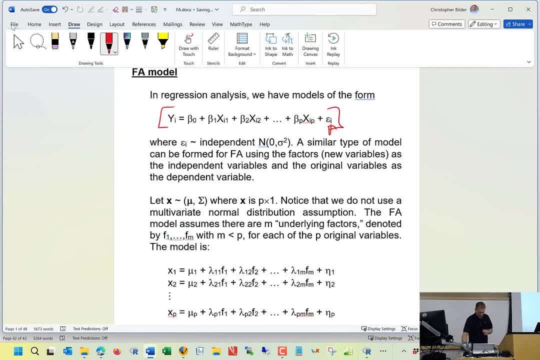 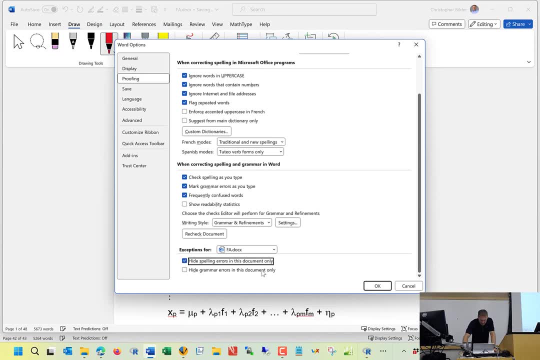 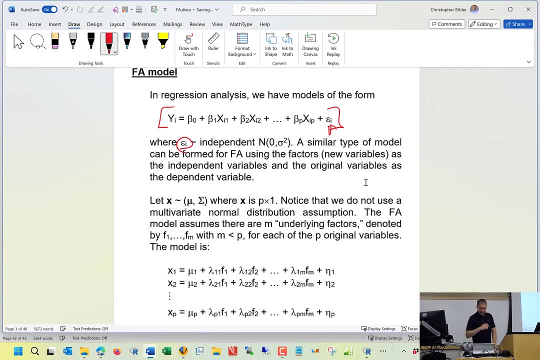 that the x's are not accounting for. Let me turn off my spell check. We don't need that. There we go Now. in this particular case, And I've said this earlier- the epsilons are unobservable random variables. They're assumed to be. 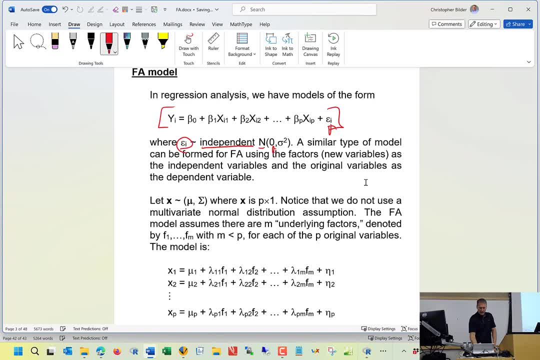 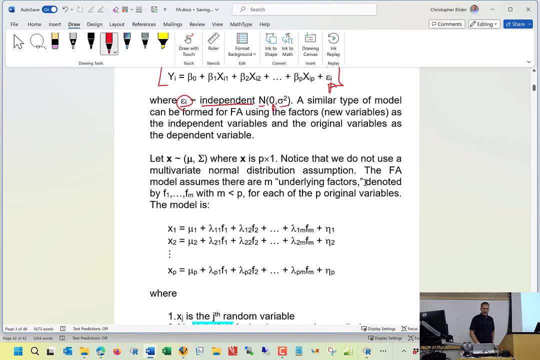 all independent, with a particular distribution, mean zero and some variance out there. Now for our model four factor analysis model. when we write it out formally, there's going to be three different representations of it and I go through the three because you're going to see all three out there In the end. we 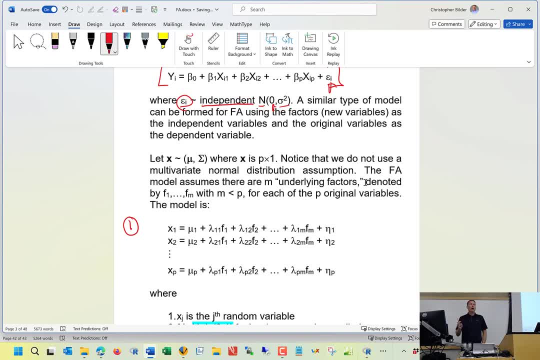 will only primarily- well, I shouldn't say only- We will primarily- use just the third one. okay, But it's helpful to see the first two because others typically talk about them and it helps us lead up to that third one. So, with our random 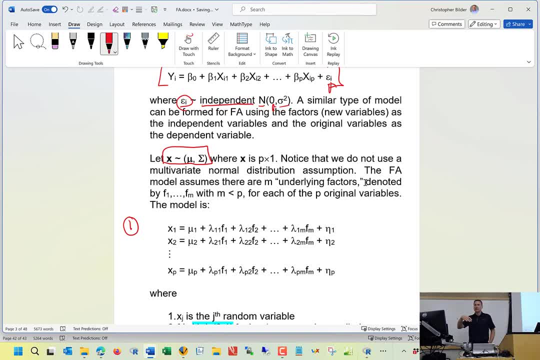 variable X, so with p variables in it. okay, We are going to assume that this random variable X, random vector x has a particular population associated with it. then there's a mean that exists, a mean vector that exists, a covariance matrix exists, but for now we are not going to make. 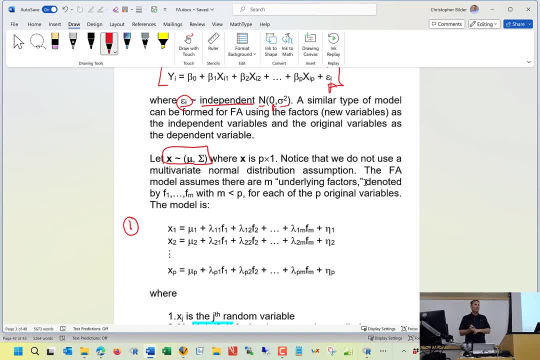 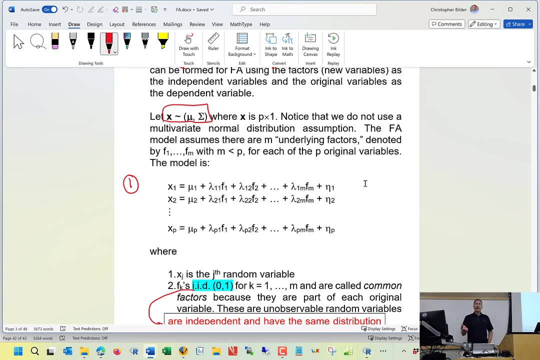 any assumptions about what the actual formal probability distribution is. We will eventually, but for now we don't need to do that. And this is what a general representation of the factor analysis model looks like. Again, think about it in the context of those test scores that we just saw. 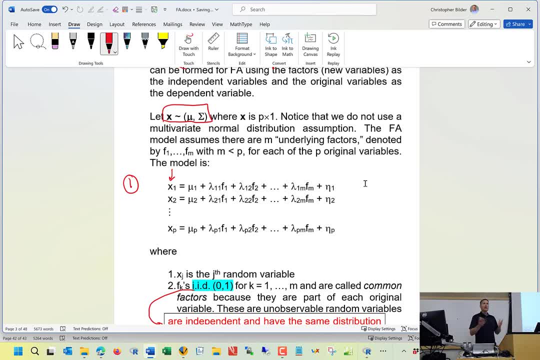 The x's essentially represent those test scores. We have maybe p different classes for these test scores And I'm going to relate x to common factors and specific factors in the following way. First, Suppose x1 is equal to, let's say, some overall mean mu1.. 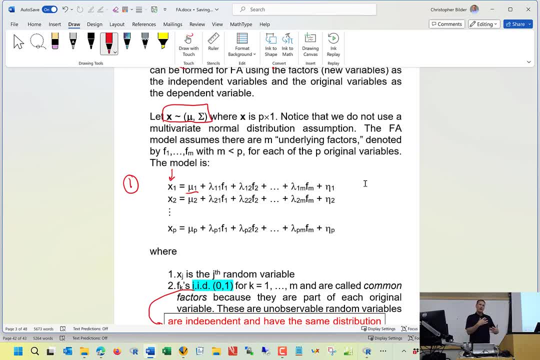 You will see how we get rid of that shortly. And then we look at deviations from this overall mean. These deviations are represented by my common factors. I'm going to have, let's say, up to m different common factors. Each of them has a corresponding lambda weight with them. 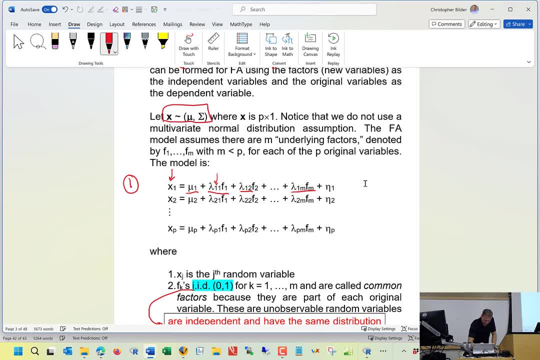 Pay special attention to the subscripts here. So the first subscript is for the original Original variable, The second subscript is for the. which common factor are we talking about? Then, at the very end, we have our specific factor And notice how that first one that just circled is eta1.. 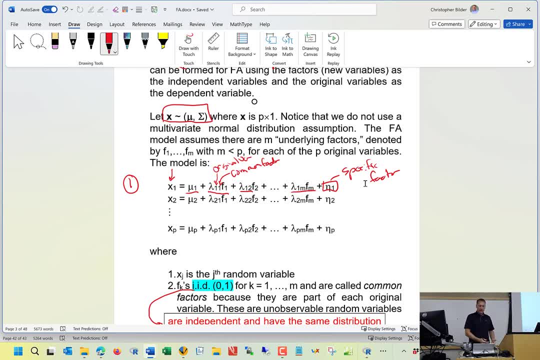 So it's the specific factor for x1.. Okay, Then x2 is written out in the same way. I have an overall mean Notice. now I have a subscript 2 on that first lambda, because this is for the second original variable, A subscript 1, meaning that this is for the first common factor. 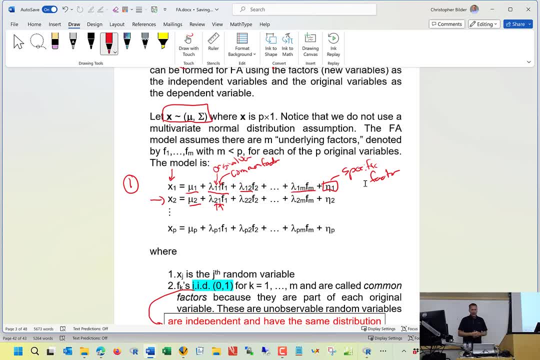 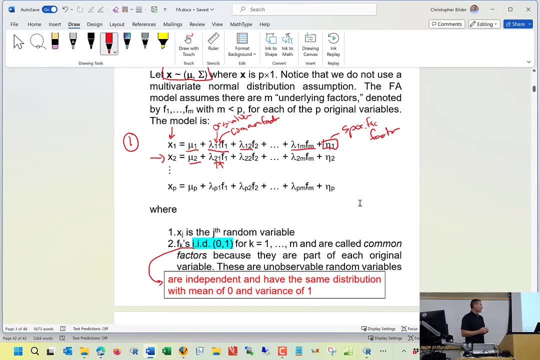 And so this is what our model looks like. So these f's are random variables, And just to maybe simplify some of the terminology, I end up using an abbreviation called iid there. Maybe you've seen it before. It's used more often in a mathematical statistics course. 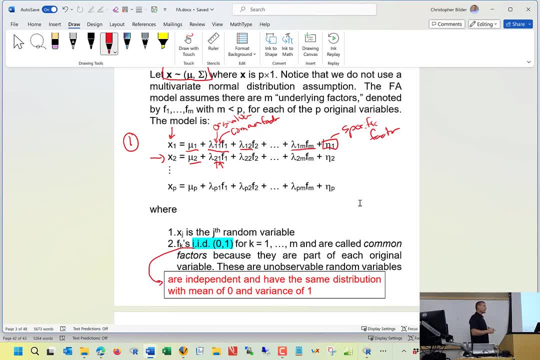 I just decided to say no, I probably didn't need to use that terminology. We're going to say that these f's are independent and have the same distribution, Each with a mean of 0 and a variance of 1.. Sorry, I didn't get that. 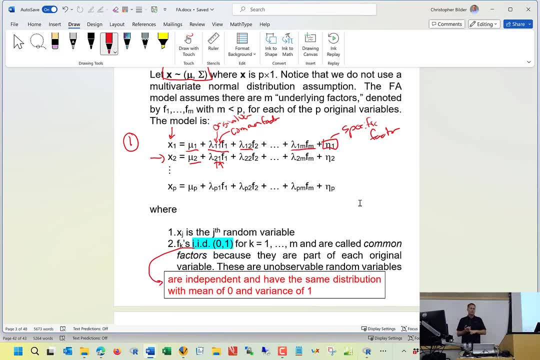 Okay. So in statistics courses you often see No. can I ask one question? Yeah, I'm sorry, I mean that lambda 1,1,. you said that first one is the original variable and the second one is the common factor. 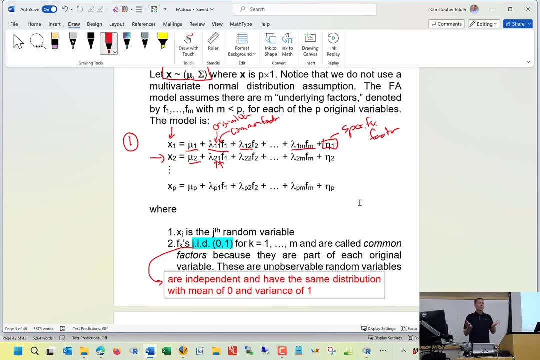 So, in comparison to the lambda f that we have in the, If lambda 1,1 is the original variable and the second one is the common factor, does that make sense? Yeah, Yeah, Yeah, Yeah, Yeah, Yeah, Yeah. 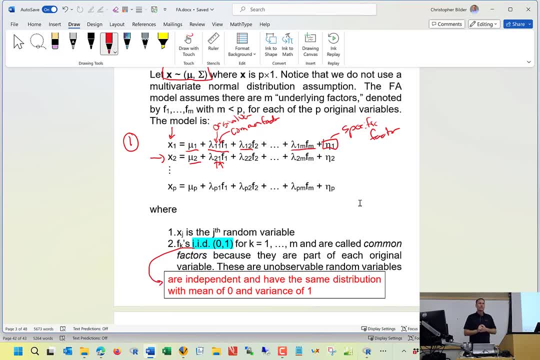 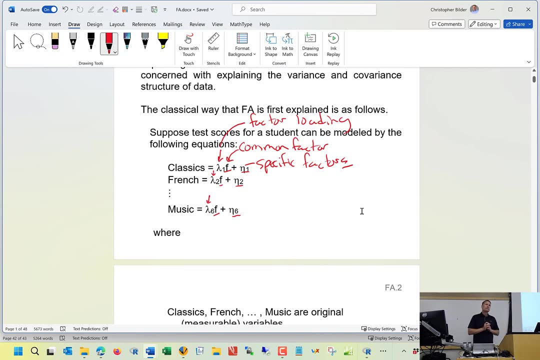 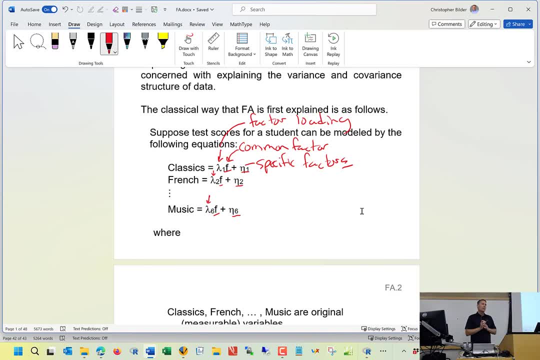 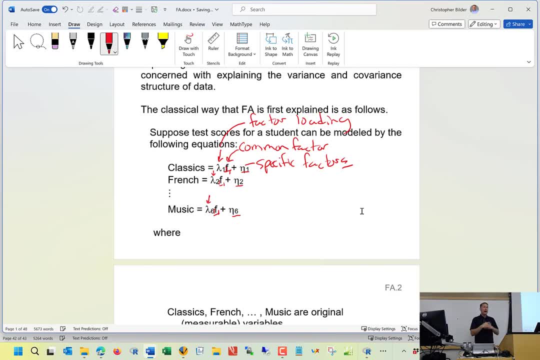 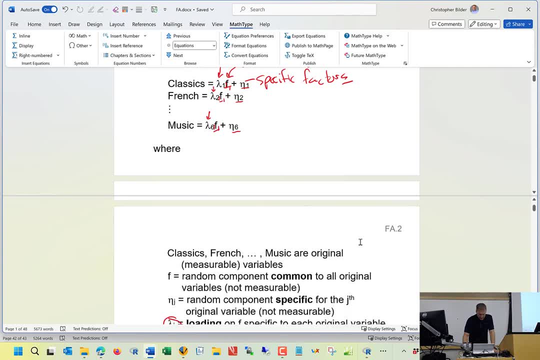 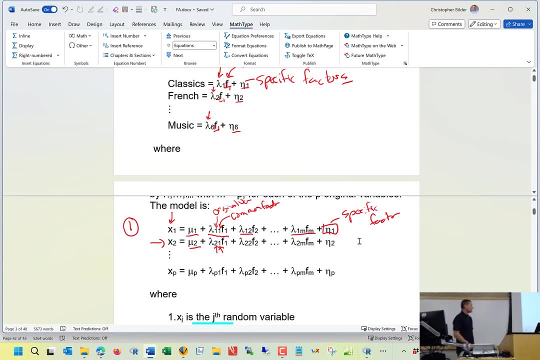 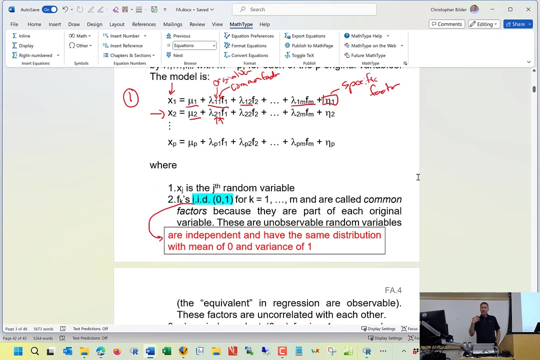 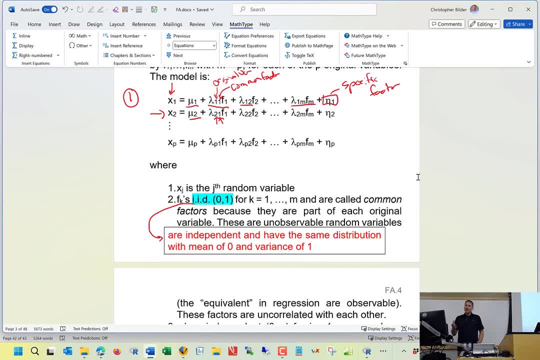 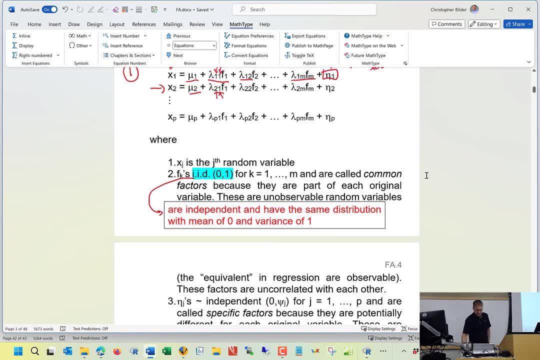 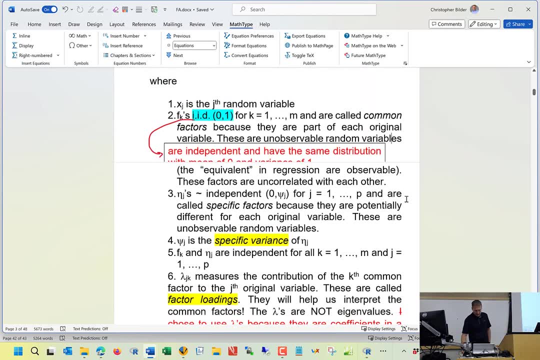 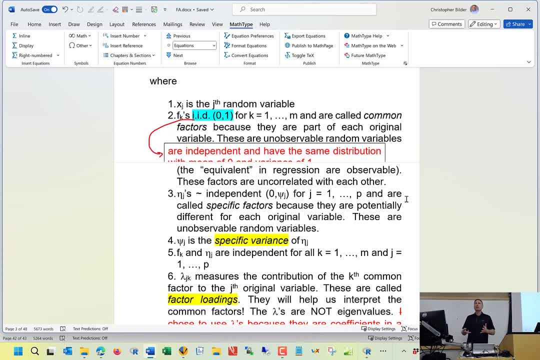 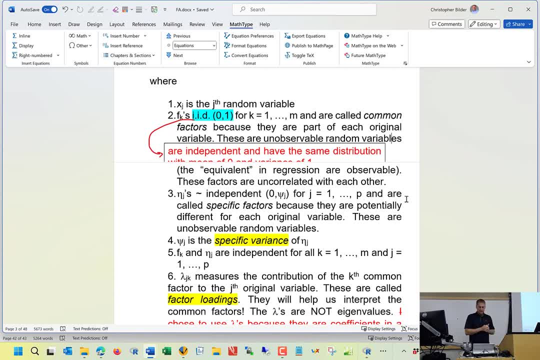 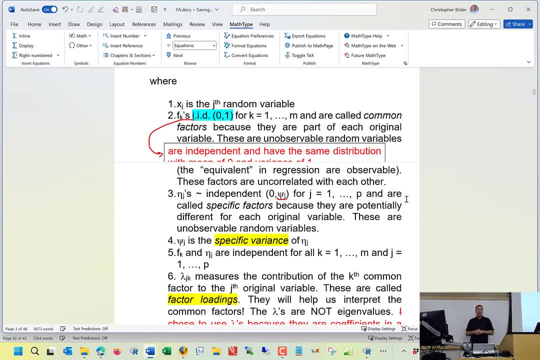 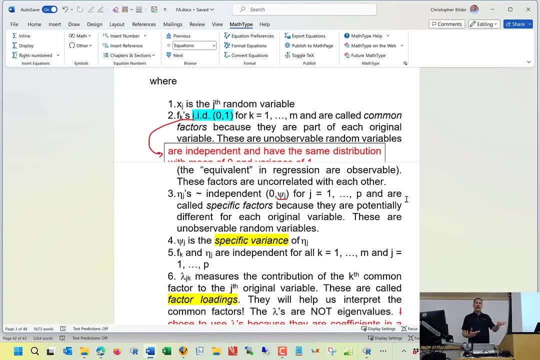 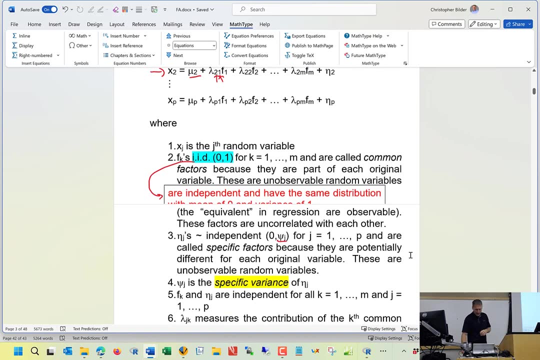 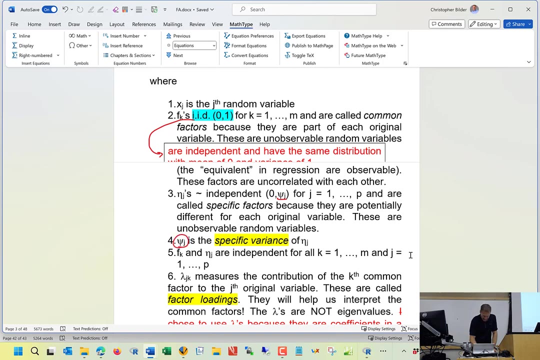 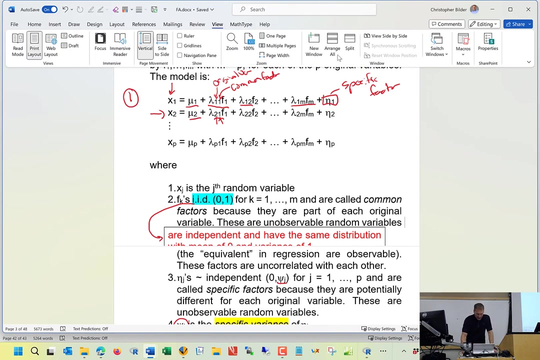 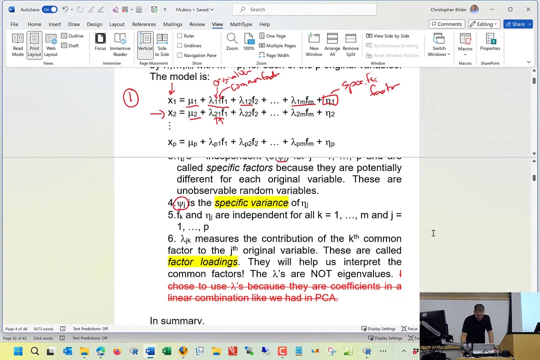 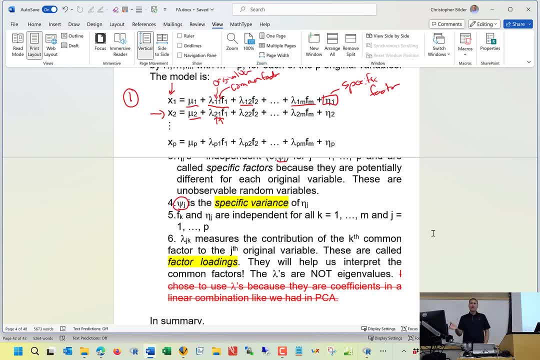 We also make an assumption that the Fs are independent of the Etas as well. Okay, Okay, These Lambdas which are weighting the common factors, I've already introduced that. they're called factor loadings, just common terminology that people use. 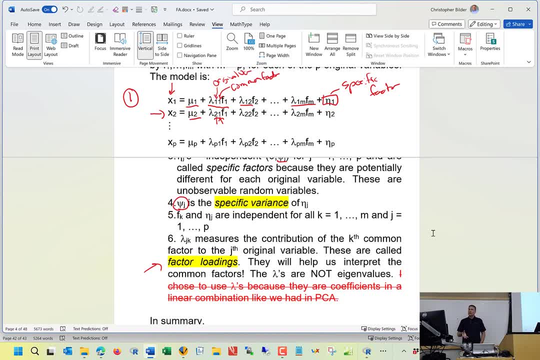 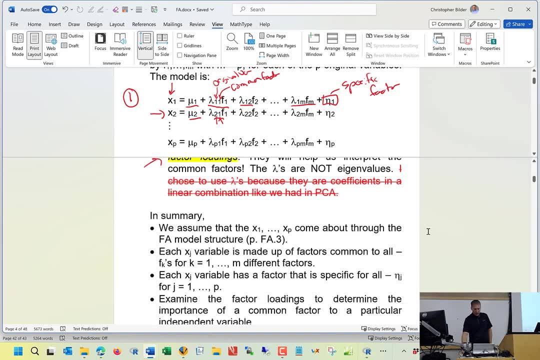 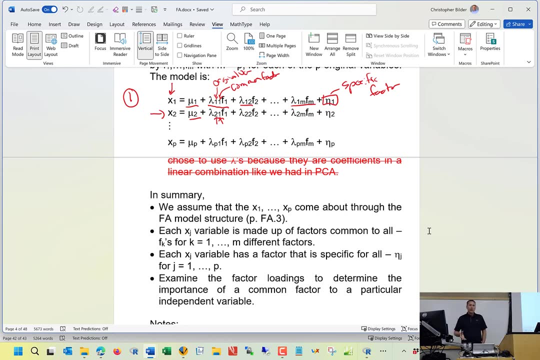 And so those Lambdas are what we're going to try to estimate. Well, actually, I actually even estimate these specific variances as well. The Lambdas will be very important to us, Just to emphasize this. You know again, if let's say Lambda 11 was 0, then that would tell us that F1, essentially. 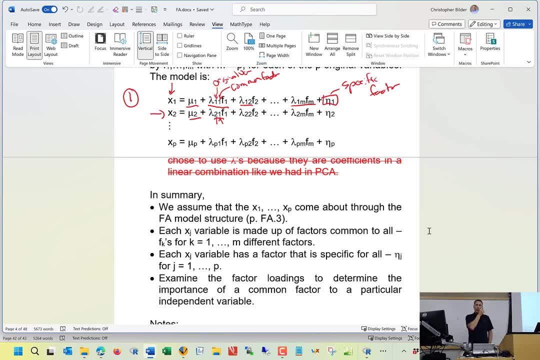 does not affect X1. And, in fact, what we will do is, for you know, look down F1. We have Lambda 11, Lambda 21, down to Lambda P1. What those Lambdas are will help us interpret what F1 is representing in terms of our original. 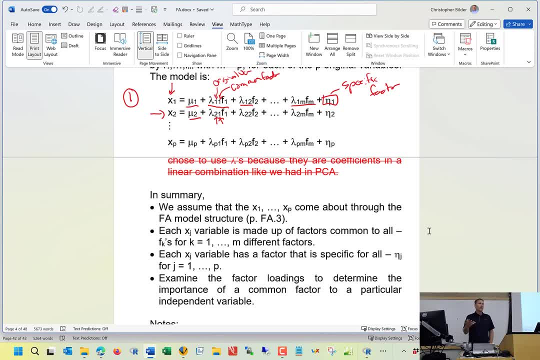 variables. So if a Lambda, Let's say if Lambda 21 was F1.. If Lambda 21 was positive, Lambda P1 was negative and they're far from 0, then that tells us. okay, you know what the common 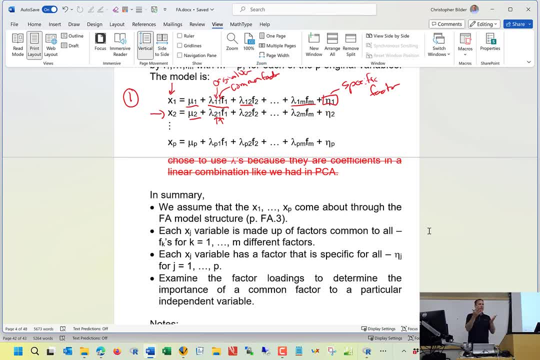 And let's say also, Lambda 11 was 0. That would say that we essentially have a contrast between X2 and XP for what this common factor is representing. This is the same kind of way that we interpret the eigenvectors before We're going to use that same process here. 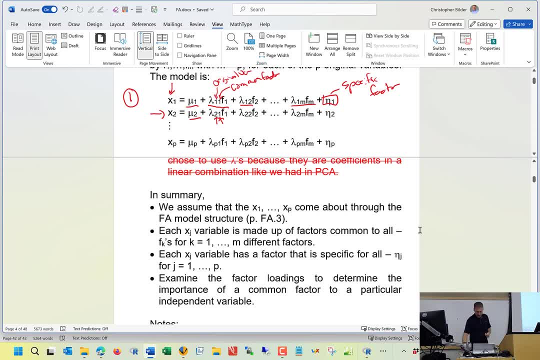 Okay, Let's see here. Yeah, Speaker 3, I just want to In the third one, the third Speaker 3, Help me out. What do you mean by third Speaker 3, It was like definition thing you talked about. 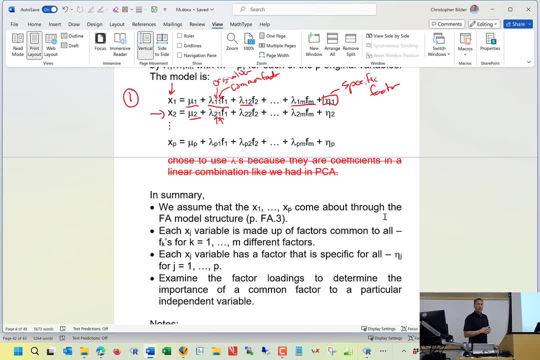 Speaker 3: Okay, yeah, I see it. Speaker 3. It says that equal to independent row. I don't understand that. Let me think. Speaker 3. So we're going to do that. Let's see here. Okay, So we're going to. 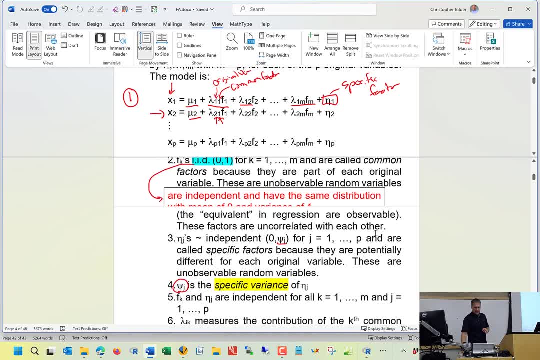 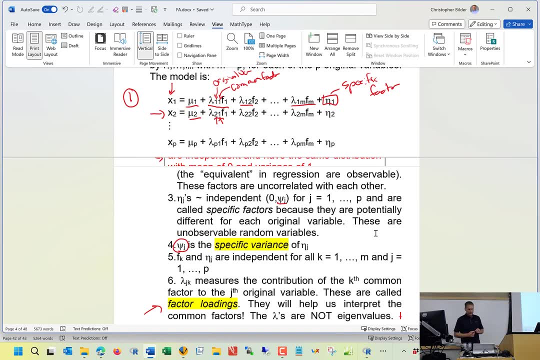 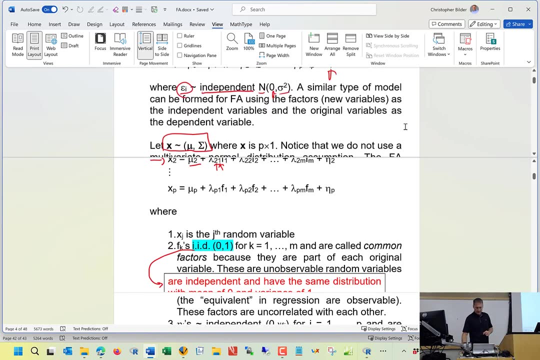 Let's see here. Yeah, Speaker 3. Yeah, Let's see here, Let's see here. Yeah, we're going to do Let's see. Yeah, Let's see here, Let's see here. than that part What this is saying. well, let's relate it to a regression model, okay, 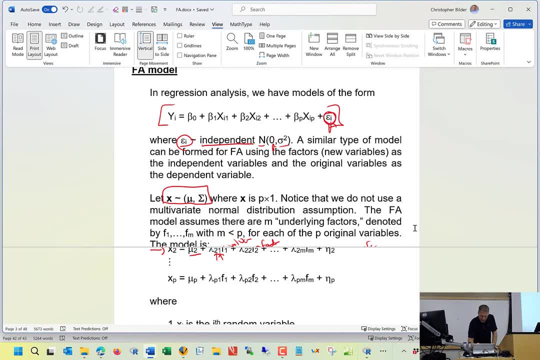 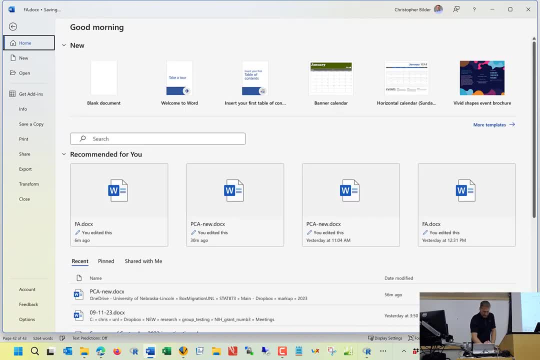 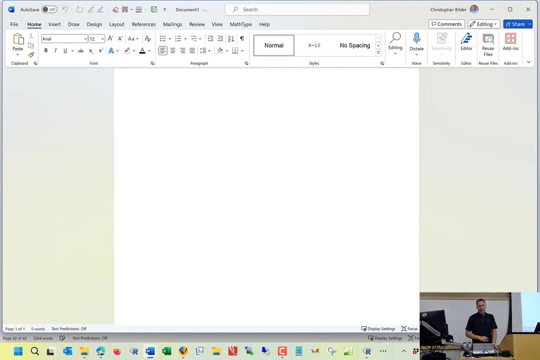 So the common assumption for each of these epsilons is that they are each independent, And so if we think of, let me actually get a new document here that I can write on. So if you remember from my introduction to R notes, you know we 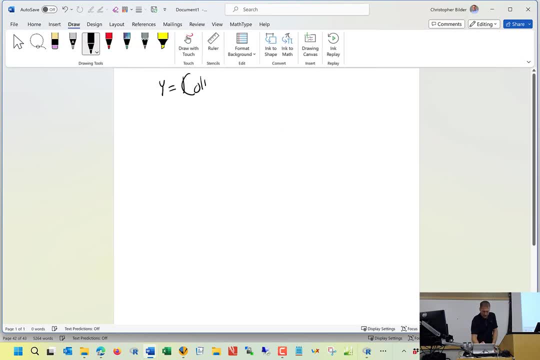 had Y was college GPA and X was high school GPA, And if one wanted to, one could write out a model for that And I'm going to put a subscript I there to represent, let's say, the Ith person And what this is. 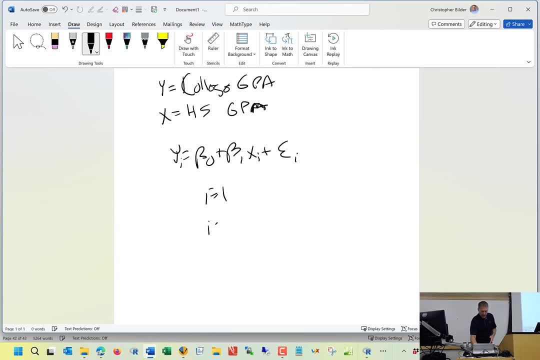 saying is that if you want to write out a model for that, you're going to have to write out a model for that, And what this is saying is: let's say, for I equal 1 and for I equal 2, person 1, person 2, what their grades are for high school and college- are not affected at all by person 2's grades. They are independent, And essentially we were saying the same thing here with respect to what these specific factors are representing. 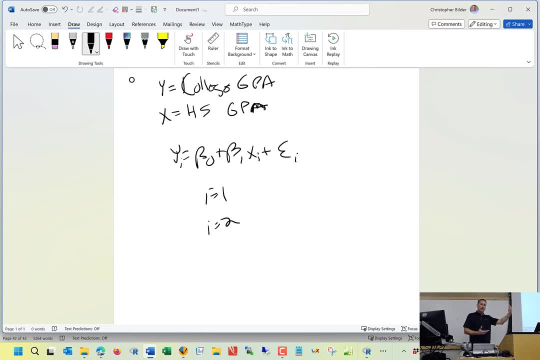 And what 801 is giving us is independent of what 802 is giving us. Okay, that's where that comes from, And you know, obviously, you know these are assumptions. You know we can think from the high school and college GPA example: well, where would this be violated? Well, let's say, you know, you have two students and one student cheats off the other student. Well, now their grades are connected and you don't have that independence anymore. 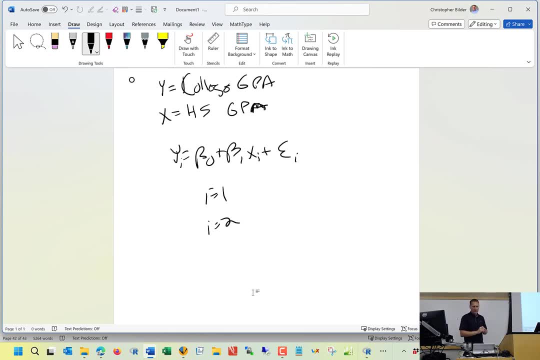 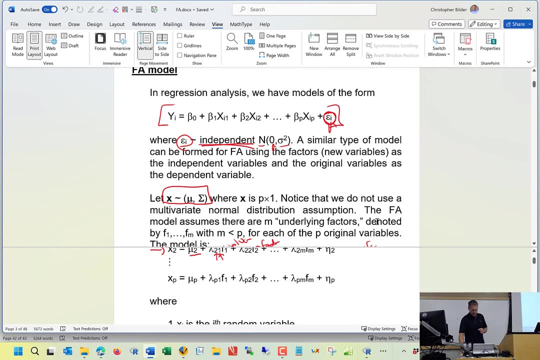 Why do we don't have the N as a background? Because for that, for the second one, because for the regression one it's like N, 0, sigma 2, but for here it's just like 0 and that. 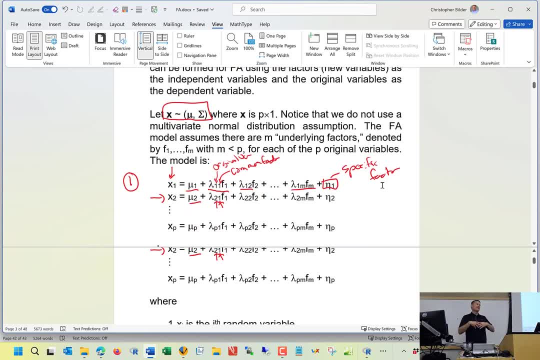 Yeah, so again, the N represents it's a symbolic way to say: I have a normal distribution. For me to write out this model, I don't actually need to make an assumption about a probability distribution. All I need to say is that, okay, I have a mean that exists. 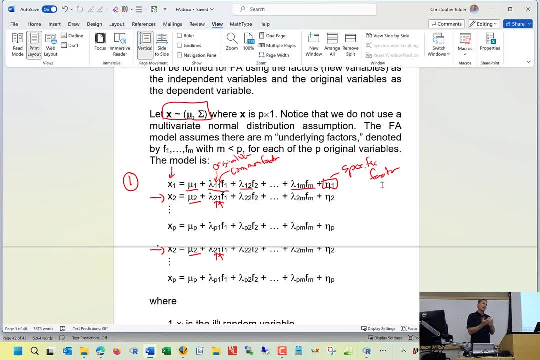 And I have a covariance matrix that exists, But I don't need to say this has a particular probability distribution. Eventually, though, when we actually do the estimation, we will actually make an assumption that I do have a multivariate normal distribution. Okay. 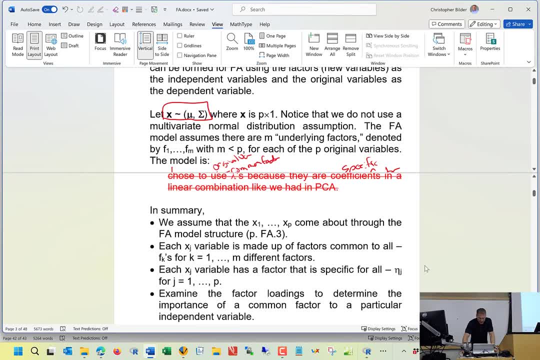 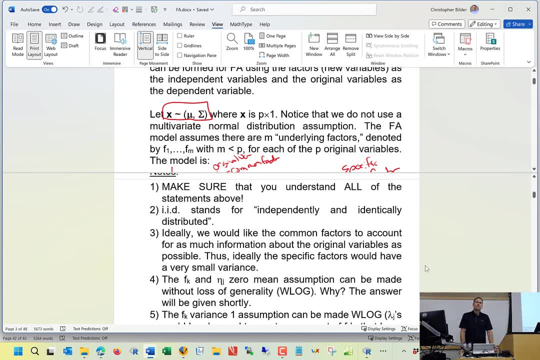 Okay, I have a question. Sure, What was the difference between factor loading and? I feel like there's. is there some matchup? The similarities are that, you know, the lambdas here are not eigenvalues or any kind of corresponding eigenvector. 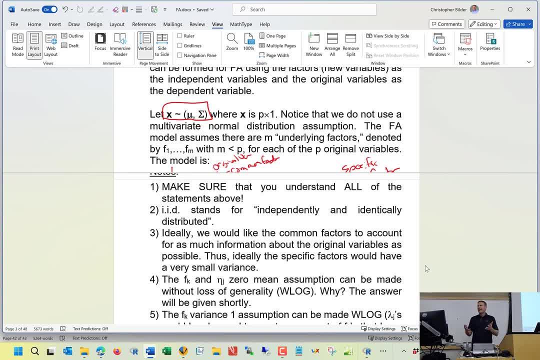 They are not. You know, I ended up using lambdas Here. maybe I shouldn't have, because these are. this is how it's commonly represented. You know the you know for. let me back up a second. 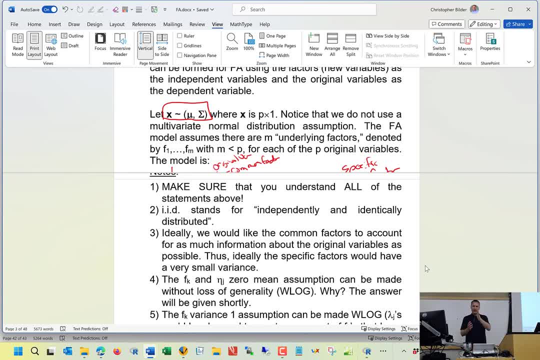 So once we got past, let's say, the graphic section, basically each of these new subsections of the notes will be essentially independent of one another. And so, while, in principle, component analysis, we did kind of continue using lambdas for eigenvalues and eigenvectors, 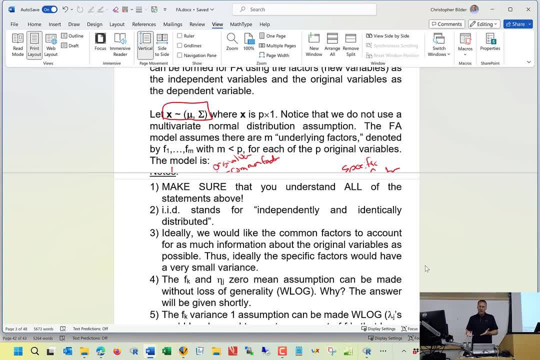 Now for factor analysis. we're not. You know why was another reason why I use lambdas Very often: when people write out linear combinations of things, they often use lambdas And that's how that notation got used. So I apologize that it can be a little bit confusing. 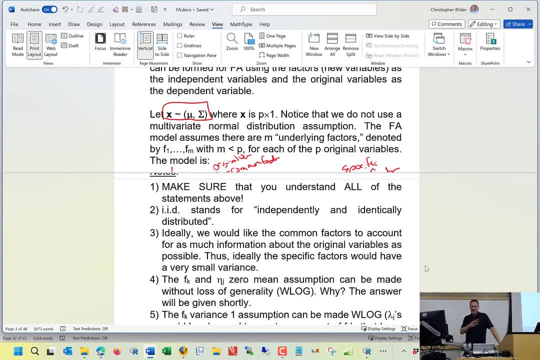 But just realize here: lambdas are not eigenvalues. That's the main thing you need to realize. here They're just always. I was going to say, Well, no, I guess that's the easiest way to put it. How about you ask that question again, if there's still, if that question still exists after we do a little bit more okay. 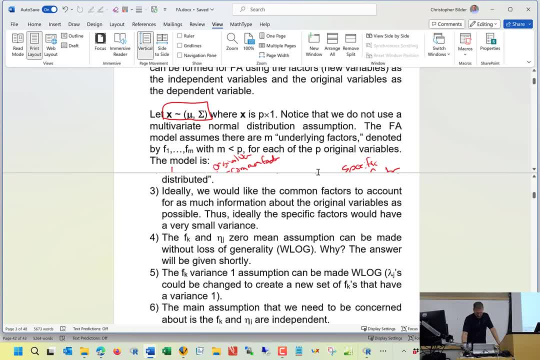 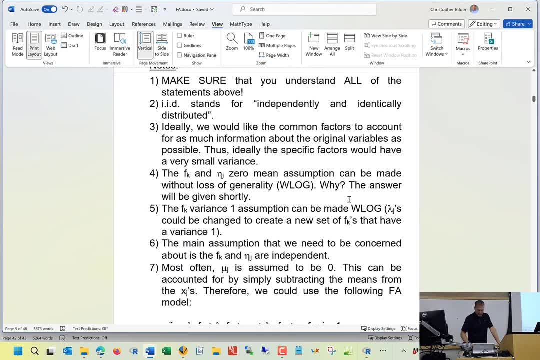 Let's see, Okay, So, So Similar to our principle components. You know, we want these principle components to explain as much information about the original data as possible, And we want to have as few principle components as possible too. Now, for us, we will want to have as few common factors as possible. 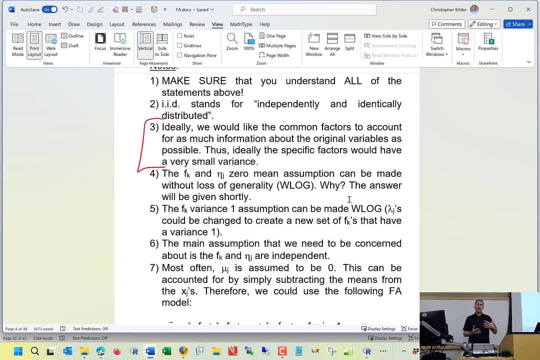 But yet still explain as much information about the data as possible. But these common factors And this information concept, though, will be defined just a little bit of a different way, Where we look at the entire covariance matrix, And you'll see that very shortly- when we want to introduce something called factor analysis equations. 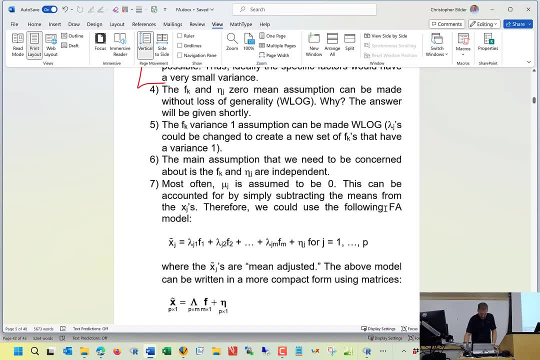 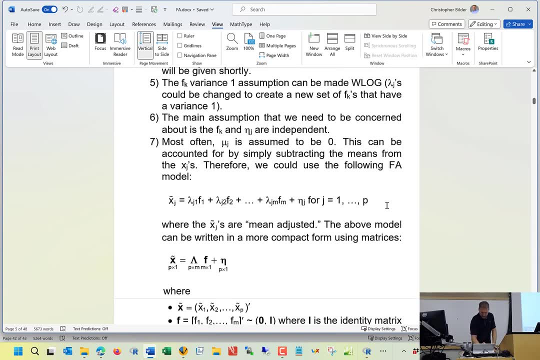 Let's see here. So I just discussed a little bit about the mathematical assumptions. You're welcome to read that some more on your own. Let's take a look at number seven. Now this you know, if you end up reading other books it can be confusing what they do with this mu. 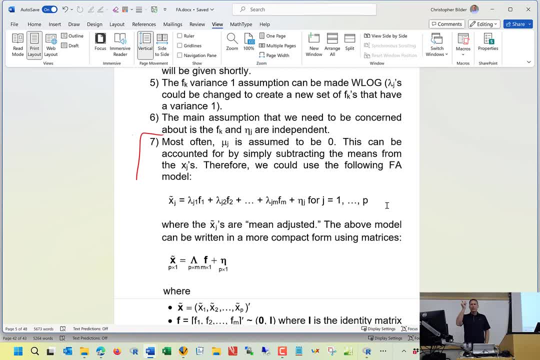 So we saw with our factor analysis model, we have this mu one, We have this mu two, mu three and so on, And some of them will not even put a mu in there. And that's because they will not even put a mu in there. 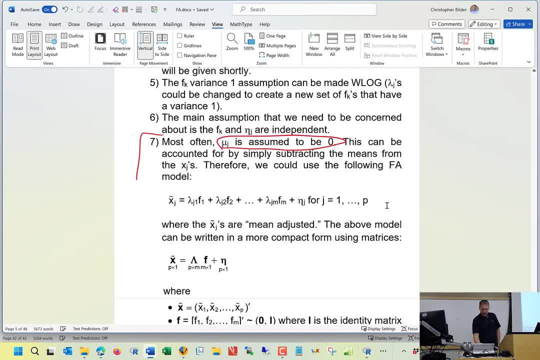 And that's because they will not even put a mu in there. And that's because they will not even put a mu in there And they will assume that the mean is equal to zero. And they don't necessarily go into details how they can make that assumption. 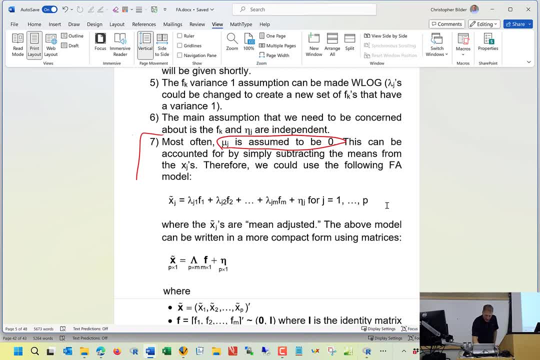 And basically all that can happen. and now this is going to be my second representation of a factor analysis model. Remember, I said there's going to be three, But we're going to primarily focus on the third one. And so the way that people can get around that assumption is that they replace our original, let's say x- the stuff that's on the left side. 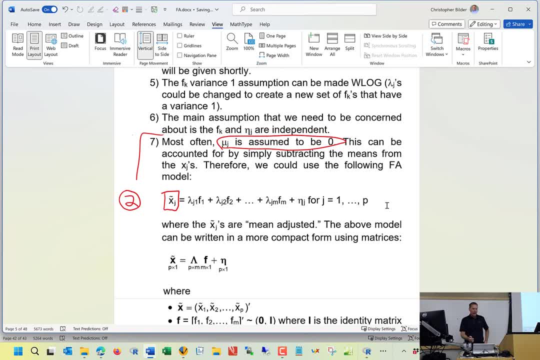 by, And so the way that people can get around that assumption is that they replace our original, let's say x, the stuff that's on the left side. So this essentially is xj minus mu j, and we could just call it, let's say, x tilde j. 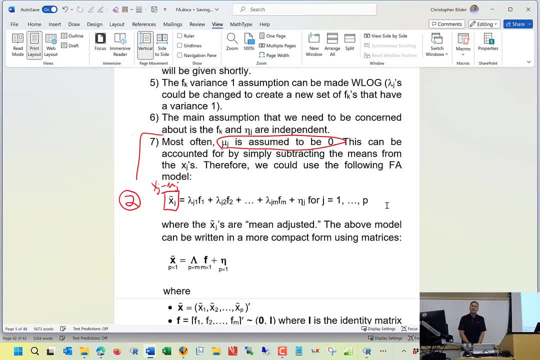 And so this essentially is xj minus mu j, and we could just call it, let's say, x, tilde j, And so that mean essentially is absorbed into the x there, in terms of it's just simply mean adjusted, And that way we don't even need to worry about the mu. 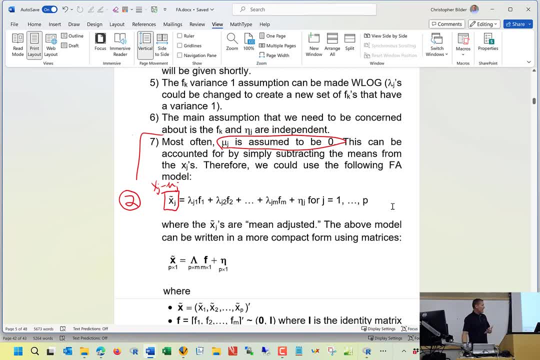 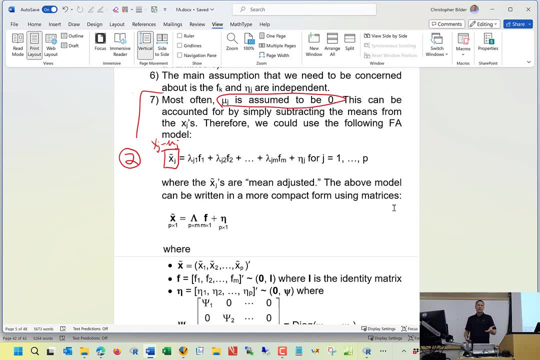 And so this is another way that you will see people get around that assumption. People represent these factor analysis models And we can also put- well, also the first model as well. We can put this in terms of matrices And notice how this makes it a little bit more compact. 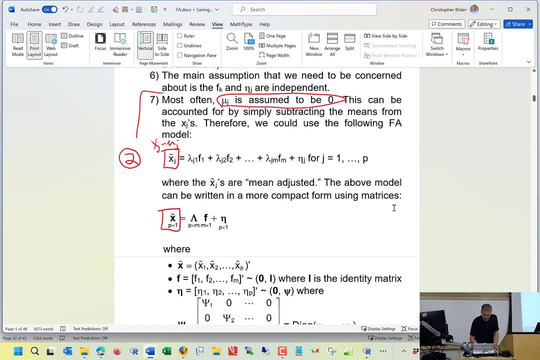 So we have this x tilde vector And then we have a matrix of all our lambdas, And so this is the uppercase greek letter lambda. then I'm now representing all of our, let's say, little lambda 1, 1, little lambda 1, 2, and so on. 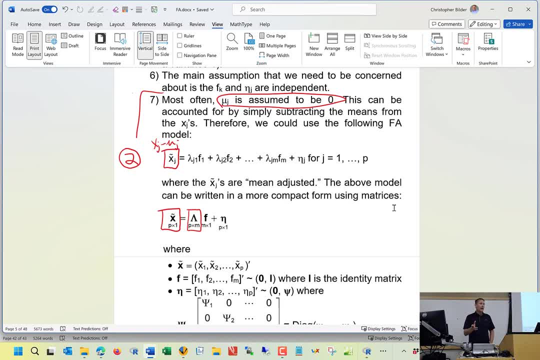 This matrix is going to be P by M Y. Remember we have in our general formulation M- common factors. It's going to be the corresponding, represented by the columns, And then we have P- original variables- represented by the rows. 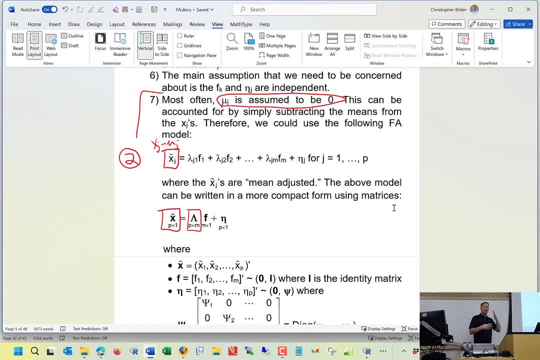 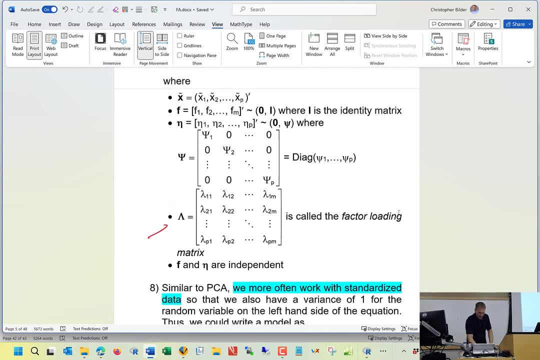 So if X tilde is P by 1, I need to make sure that I have P rows of these lambdas. So let me actually show you that. So this is what my lambda capital lambda matrix then looks like. 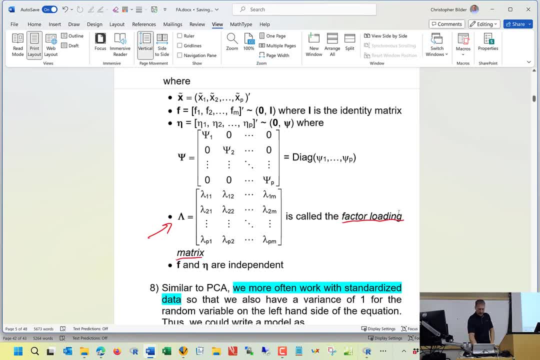 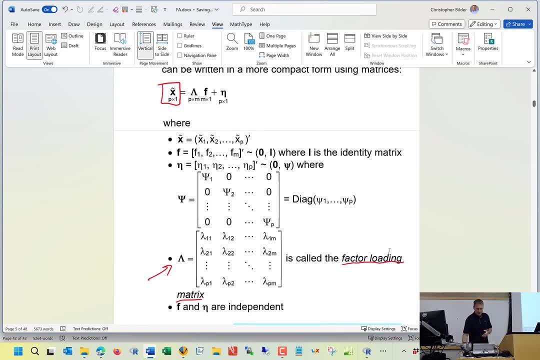 This again, there's terminology here. This is called a factor-loading matrix. Makes sense Then. then for my common factors, it's going to be M by 1 vector. So simply, you put your F1, F2, all the way down to FM in it. 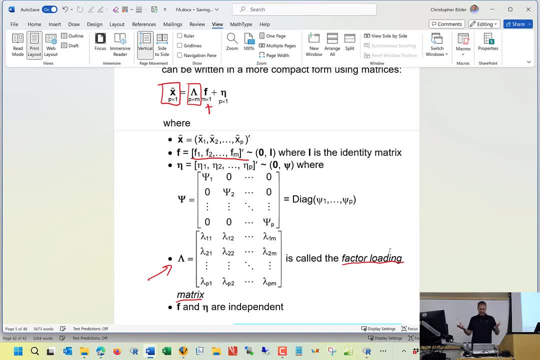 And since this is a multivariate class, then I can say: okay, well, this F has a distribution that has a mean vector of 0, and I, as the identity matrix- I'm sorry- as the covariance matrix- We've got the covariance matrix. 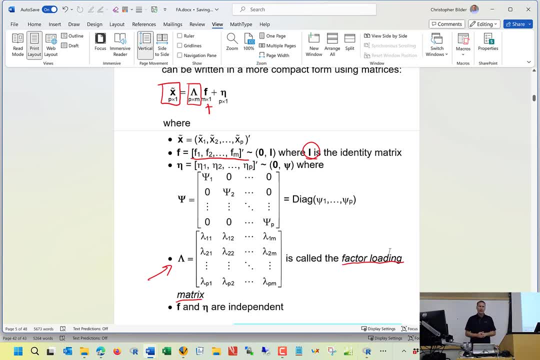 We've got the covariance matrix. We've talked about identity matrices a little bit before. Does anyone remember what an identity matrix is? Yeah, All the values on the diagonal are equal to 1.. All the off-diagonal values are equal to 0.. 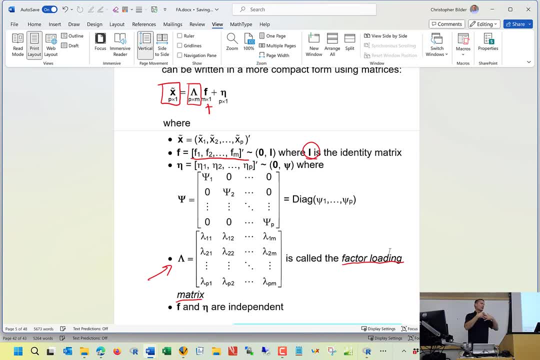 Well, why is our covariance matrix that? Well, just our mathematical assumption. with this model, each of the Fs have a variance of 1, and all the Fs are independent of one another. So, like, the covariance of F1 and F2 is 0. 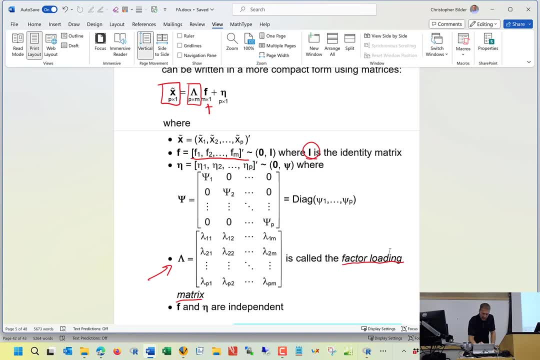 That's why, Then, we also have a vector of our etas. It has to be P by 1 as well, because, again, I have P different X-tildes And we can put these etas in the vector like that. 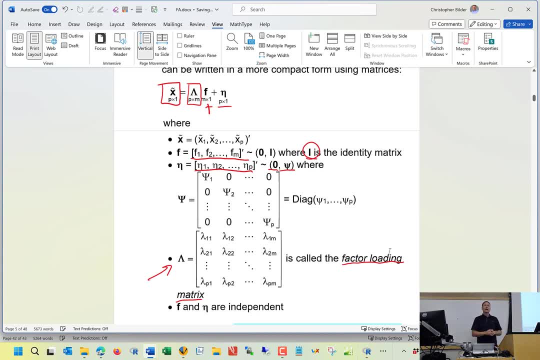 It has a distribution with a mean vector of 0 and a covariance matrix. How about we just call it eta itself And notice that that's also a diagonal matrix, where on the diagonal we have the corresponding variances. So this would be the variance of eta1.. 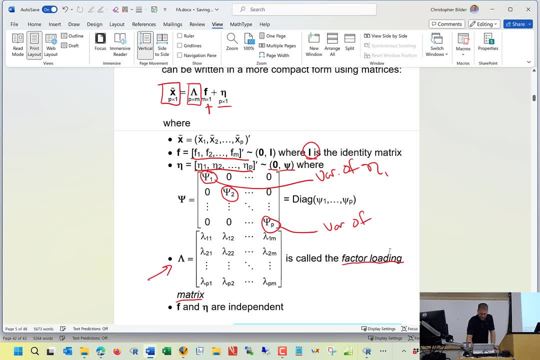 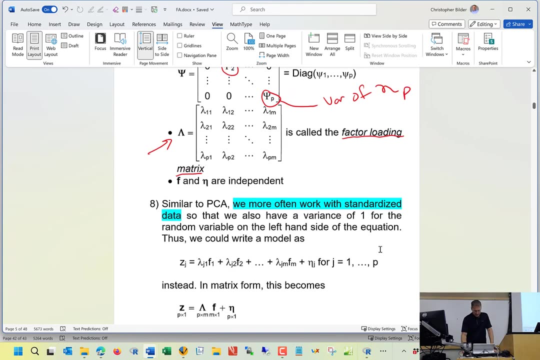 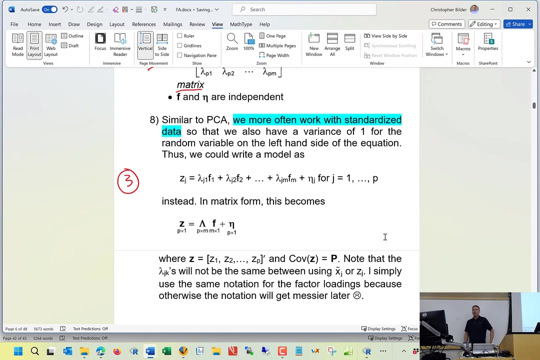 This would be the variance of etaP. These etas are assumed to be independent of one another, so that's why I have zeros on the off-diagonal elements. Okay, Okay. Now, finally, We get to the actual model that we will typically use. 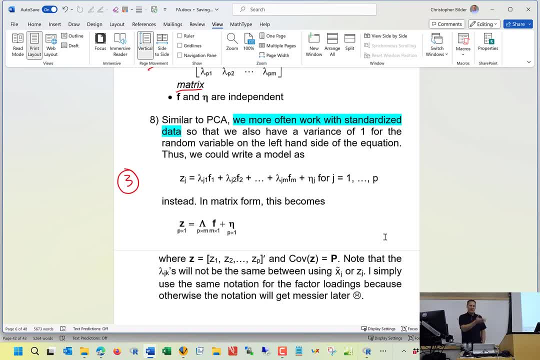 If you remember well, you should remember we actually talked about it earlier today. With principal component analysis, we typically use the. we work with the correlation matrix Or equivalently you could say the covariance matrix of our standardized variables. 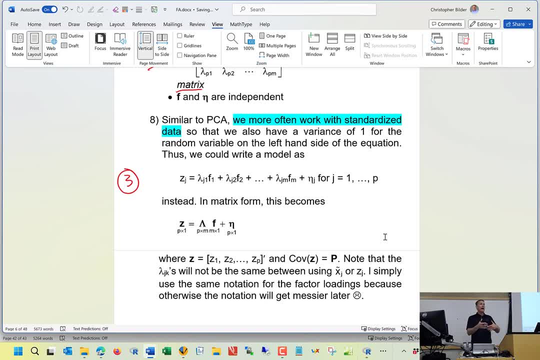 The reason being is because our variables will often have different amounts of variances or different sizes of variances, And if they are very different, that can screw things up. Okay, Similar thing here. So we will typically work with standardized variables so that z1 has a variance of 1,. 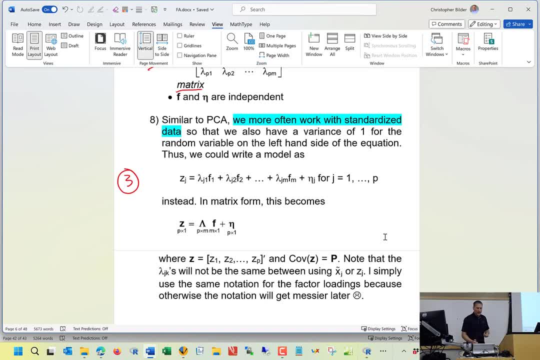 z2 has a variance of 1,. z3 has a variance of 1.. And so, finally, we get to our last representation, and this is what our factor analysis model is going to look like. So I just put a z on the left side. 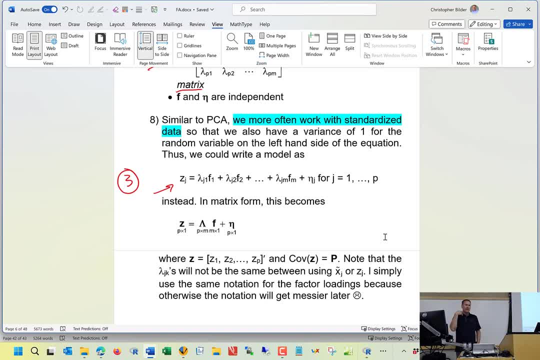 And just for emphasis, because I know sometimes this can be easily missed. So notice here: I have: j equals 1 to p. Well, what does that mean? Well, that just simply means I have: z1 is equal to lambda 1, 1, f1, all the way down to lambda 1, m, f, m plus eta 1.. 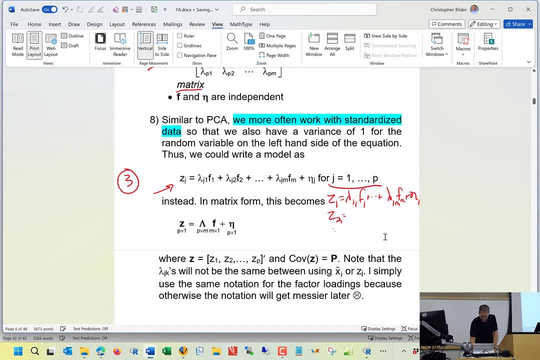 Then I have z2.. I can write it out. Now I have all the way down down to zp and I can write it out. That's what just said, just what that means. So I still have basically p different equations. 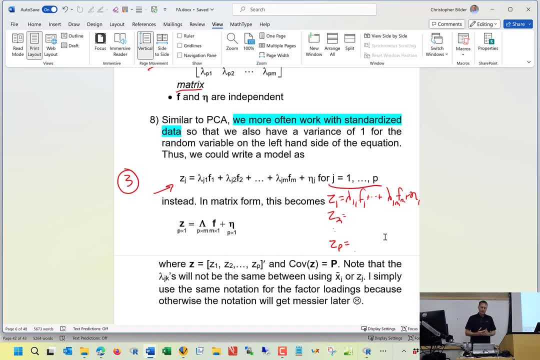 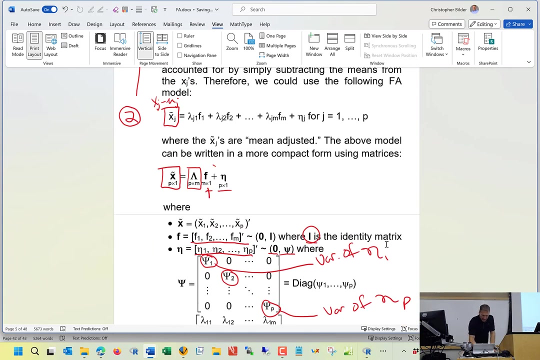 one equation representing each of our original variables. I can put all this into a matrix form here Now, just to simplify the notation terminology and stuff like that. notice that I am using lambda f and eta there and I also use lambda f- eta there. 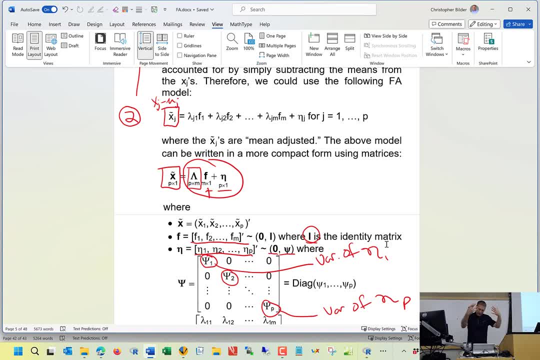 I think it will be clear. we're always going to be using- almost always- standardized variables, and so that's why, just rather than putting like I did with the principal component analysis section, putting an asterisk there to say, hey, now we're using standardized 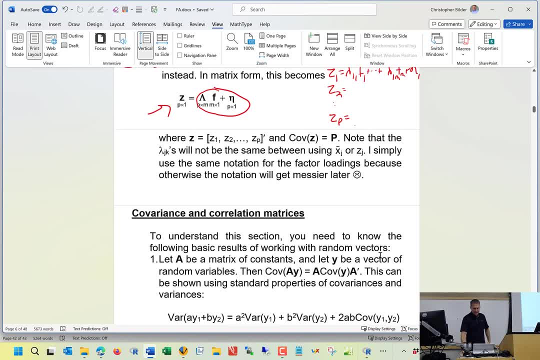 Perhaps that's why I should have just done the principal component analysis section too. So now remember, just for emphasis- this is going to come up maybe shortly, depending upon how far we get- that covariance matrix for z is equivalent to the original correlation matrix for the x's. 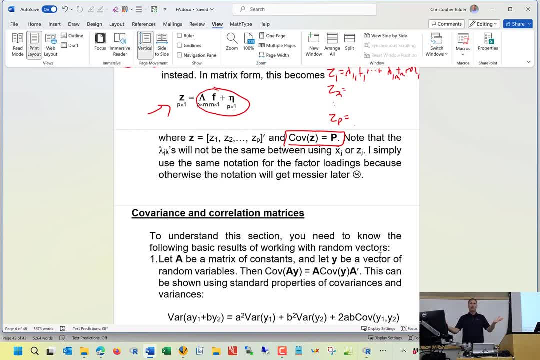 Also, you could say it's the correlation matrix for the z's as well, back from the data distributions correlation section when we saw that. So that's why we're going to have to sort of use the. or we could say we're going to use the. 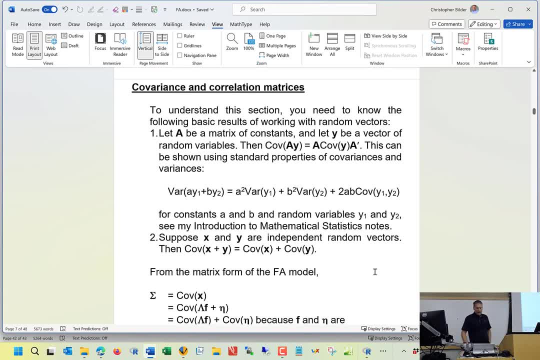 or we could say we're going to use the. we could say we're going to use the, or we could say we're going to use the correlation matrix for z. Okay, Next, Now we're going to start talking about. well, how can I estimate these lambdas? 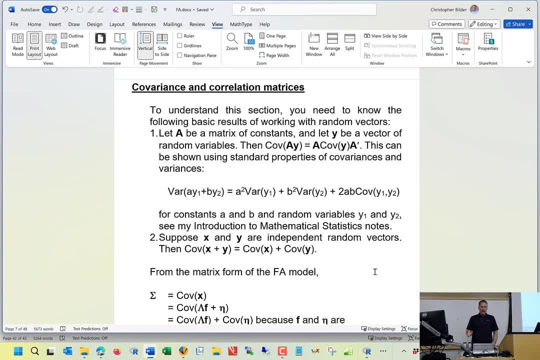 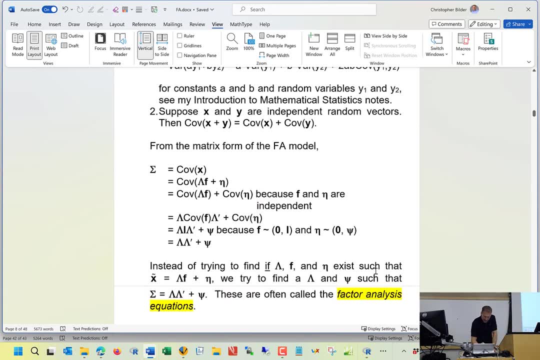 And the way that we're going to do this is false. so I'm going to just jump ahead a little bit and then I'll come back. Let's look at our original factors and let's say that we have two factors here. 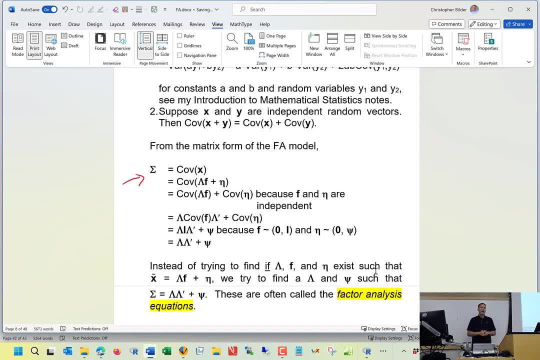 Okay, First one is the correlation matrix and then one is the derivative factor factor analysis model. so model number one, where I have it defined in terms of the x's, The covariance matrix for x, we would denote it as the uppercase Greek letter sigma. 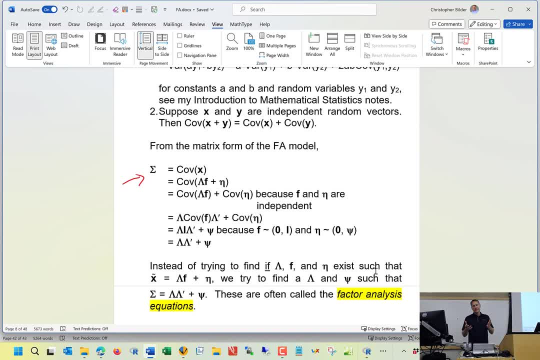 With a little, what we'll call a little bit of a deprivation. we could write this sigma as this: your factor loading matrix times the transpose of your factor loading matrix plus your diagonal matrix of all those specific factor appearances. You could write it in this form because of our model structure. 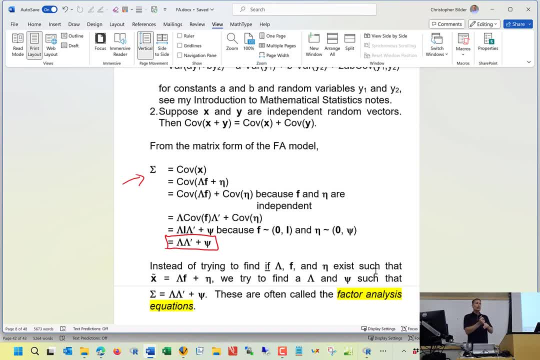 So if you somehow knew what your sigma was, you now have a way to write it. in this form, You could solve for each of your factor loadings, your lambdas and those specific variances. You could set up a system of equations and solve for each of the lambdas in each of this. 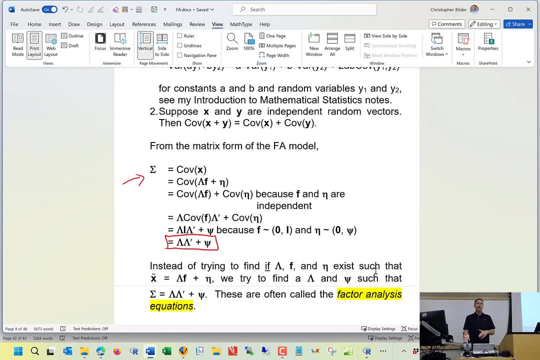 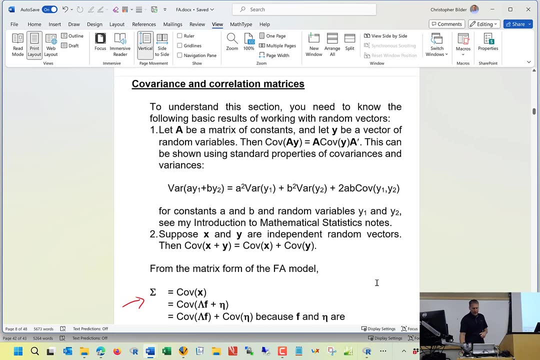 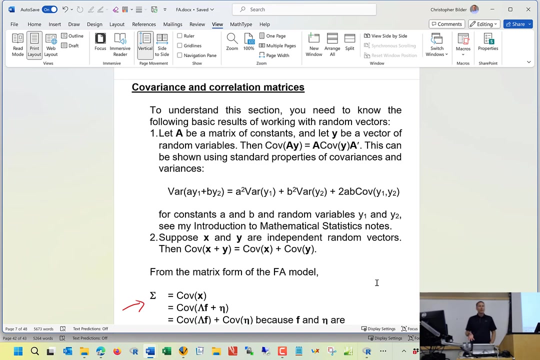 size based upon this relationship there. That's how we're going to, in the end, estimate each of these factor loadings and these specific variances. More on that shortly. Okay, So now we come to a part of the notes where it's where I have to admit it would be helpful. 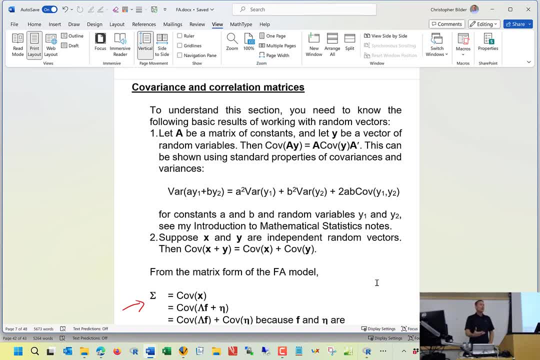 if you, if everyone, had a mathematical statistics course where you are comfortable with deriving variances, You're comfortable with deriving covariance and stuff like that, And I understand that most of you are probably not. So what I'm going to do next is talk a little bit. 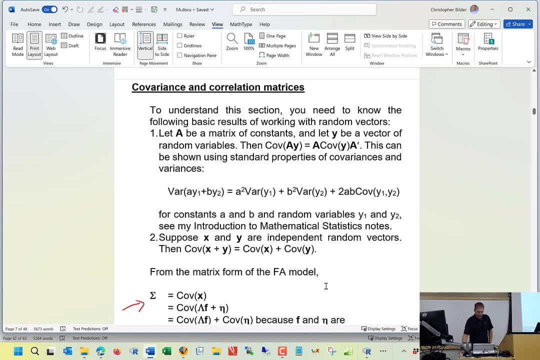 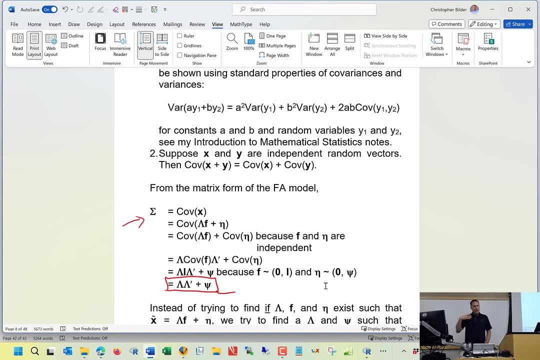 about how these factor analysis- in case I didn't say this, these are called the factor analysis equations- How these factor analysis equations come about. I'm going to give you a little bit of introduction to what the mathematical statistics part is. You are not required to, I'm not going to ask you. let me put this. I'm not going to. 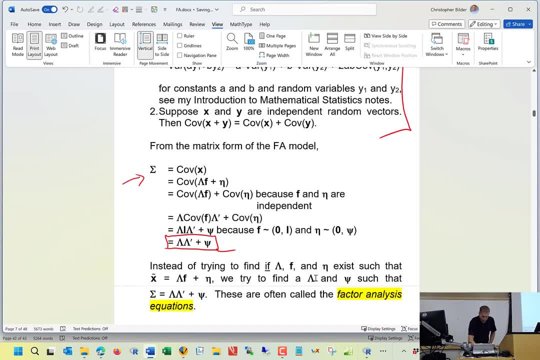 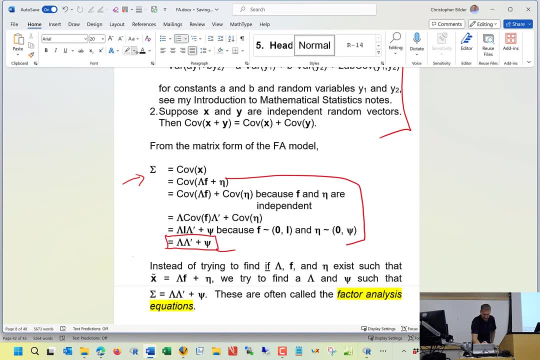 ask you a question on the test about the stuff that I just highlighted there, or the stuff that I just highlighted there. You do need to understand- sorry, give me my highlighter- You need to understand what I just highlighted there, That this relationship exists. 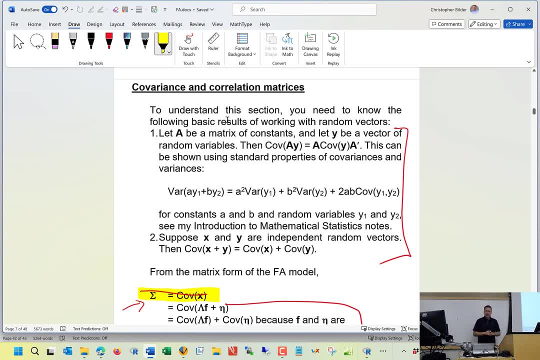 Okay. Now if I wanted to, let's say I'm going to do this, Okay, I'm going to do this, I'm just going to do this, I'm going to do this to, let's say, find the covariance matrix of 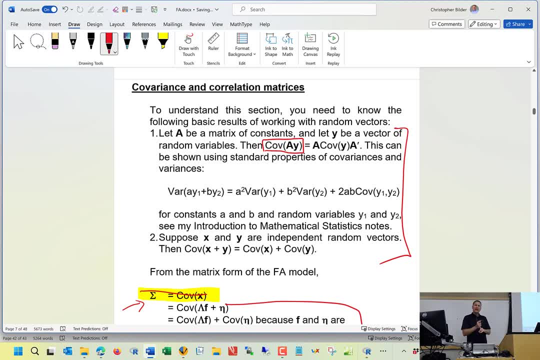 if I have a random vector, call it y, and a matrix of constants, call it a. If I wanted to find the covariance matrix for that, that ends up being a times the covariance of y, a prime. Now, why would this be important? 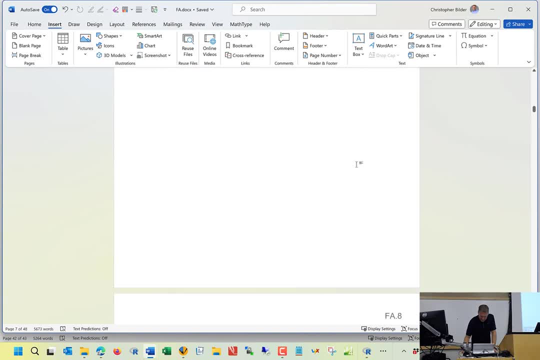 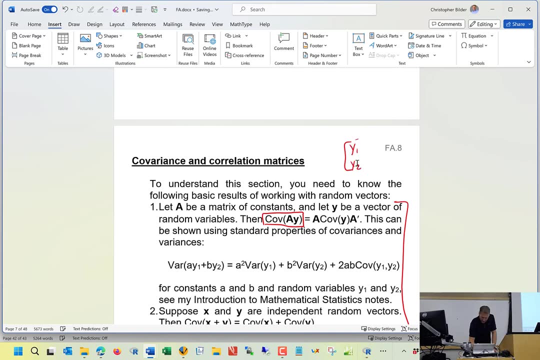 Let's say: let me remove that. Let's say that I have a two by one vector for y. It has components y, one, y, two. And let's say that a looks like this: Oh, it's one negative one, zero and one. 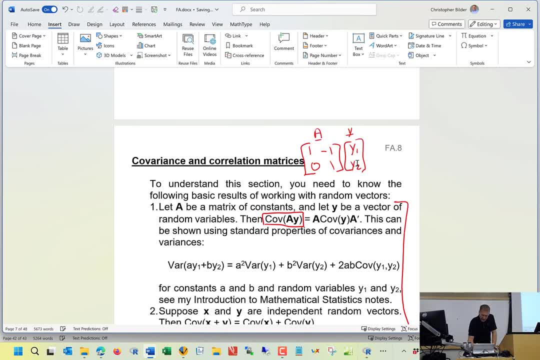 So that's my a, Here's my y. Now, if I do the math here, I end up getting y one minus y two, and then just y two. So this matrix of constants- let's call it that a- allows me to find linear combinations. 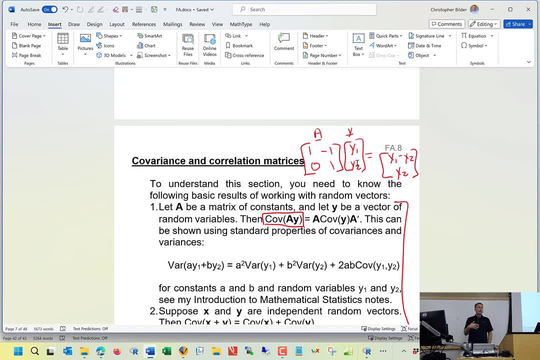 of my values of my random vector. This frequently occurs in statistics. So, for example, if you've taken like a STAT 802 course, which is our experimental design course, and you see this a little bit in STAT 801, but we don't, 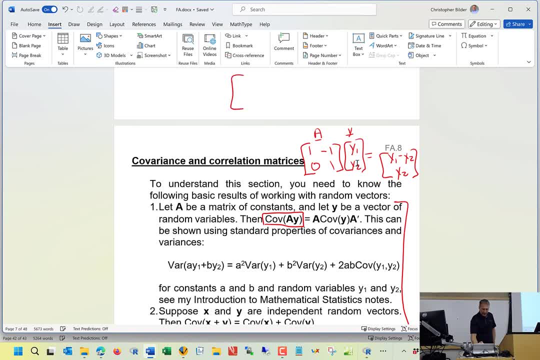 we just introduce it from a matrix perspective. You know, let's say if I have a vector of mu one we'll do mu two, mu three. So you know, often in those kinds of classes you're interested in doing analysis of variance methods. 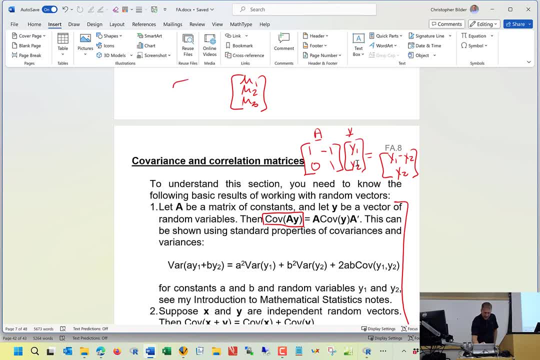 You want to find differences amongst means, And let's say that I have a matrix that looks like this. This ends up being mu one minus mu three, Mu two minus mu three. You know that should look a little bit familiar. You're comparing all pairwise differences of means. 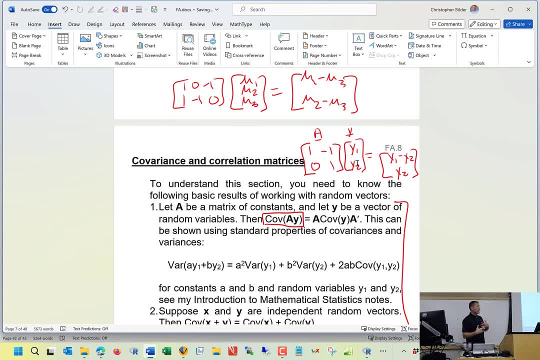 And the way that you can get that is through a representation like this. This is like my A matrix, Okay, And so, in order to derive, then let's say, if you wanted to, let's say a confidence interval for mu two, I'm sorry, mu one minus mu three. 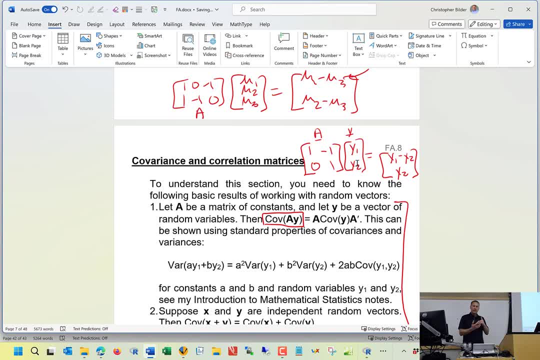 In order to derive that, you would often have to start with the estimated covariance matrix for the corresponding sample means, And then you could apply this A matrix with it to find the corresponding variances that you need for mu one minus mu two and mu one minus mu three. 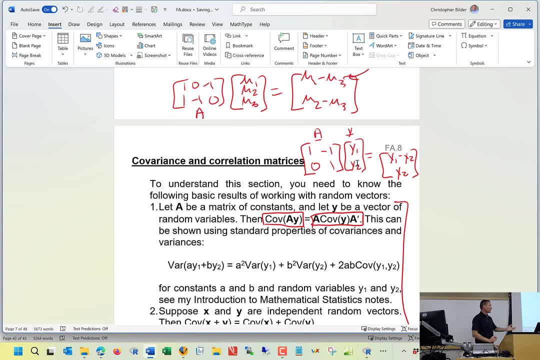 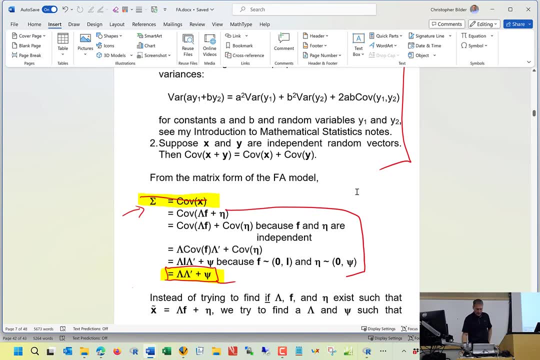 without going into too much more detail, And this can be easily found through this little relationship there. Okay, Now also, if I have, let's say, two random vectors, let's call it x and y. If I want to find the covariance of x, 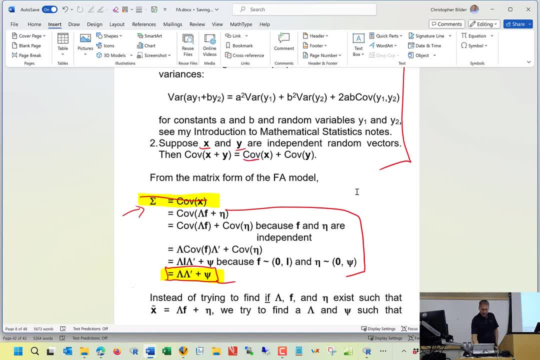 plus the covariance of y, if they're independent. I can just find the individual covariance matrices for x and y and add them together, And hopefully that makes some intuitive sense If one doesn't affect the other, okay. well, that's all you need to do. 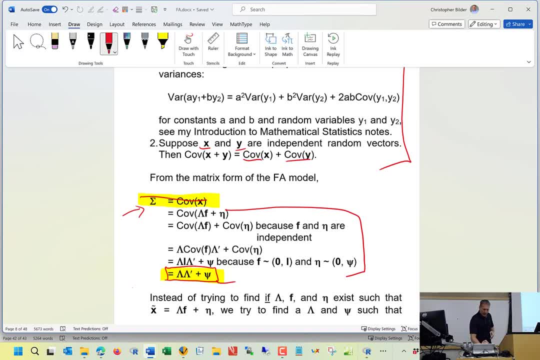 So why is this all important? Well, it's because this is it's going to give us- I guess you could say- a little background about how this expression for sigma comes about. So sigma's just another way to represent covariance of y. 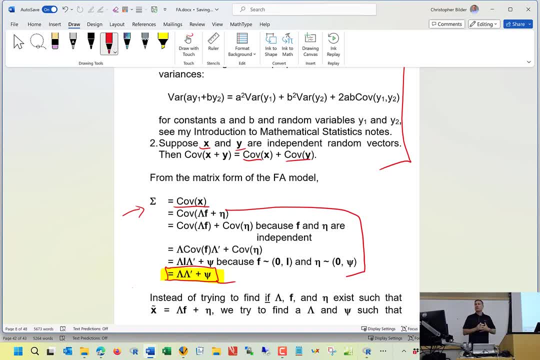 covariance of x. You know, we saw this first in the data distributions and correlations section. Well, what is x? Well, with our factor analysis model, this x is actually lambda f plus eta. Okay, So I can simplify this. Remember how f is equal to lambda f plus eta. Okay, So I can simplify this. Remember how f is equal to lambda f plus eta. Okay, So I can simplify this. Remember how f is equal to lambda f plus eta. Okay, So I can simplify this. Remember how f is independent of eta. 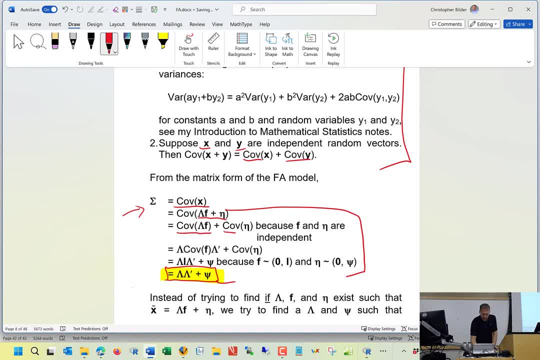 So that means I can then write it as covariance of lambda f plus the covariance of eta, just applying number two right there. Then how about I just write out this covariance of lambda f, write it out in terms of just the covariance of f? 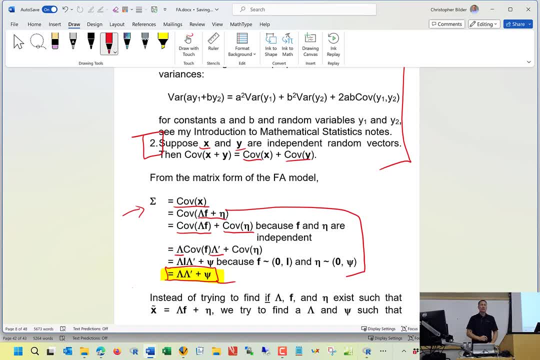 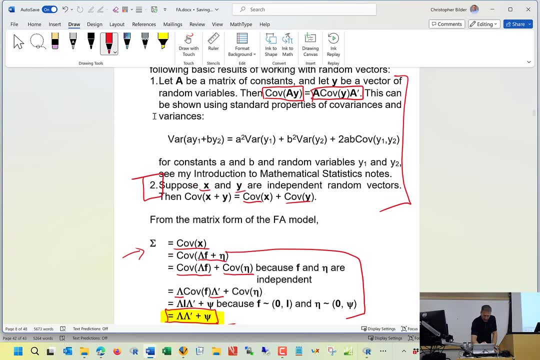 So I can factor out my matrix of constants, those factor loading matrices, by applying. you know what was above by applying. you know what was above by applying. you know what was above by applying number one there. 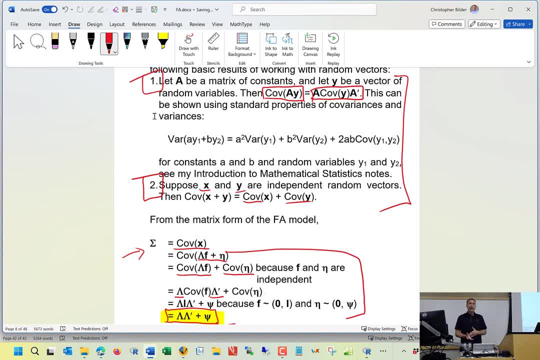 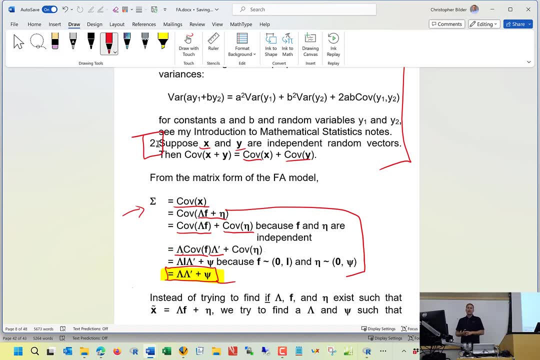 So this lambda is essentially a, The y is f. What is the covariance matrix of f? Well, we just saw that about 10 minutes ago, Remember, we assumed that they each have a variant, each of the f's, each of the common factors. 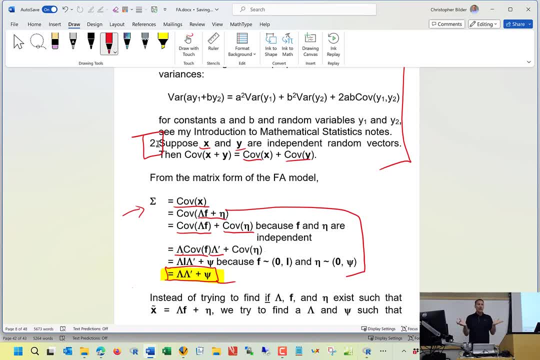 have a variance of one and they're all independent. So I have an identity matrix. That's the covariance matrix for f. So that's what this represents. It represents right there. And of course, if I take one matrix times the identity matrix, I get that one matrix back. 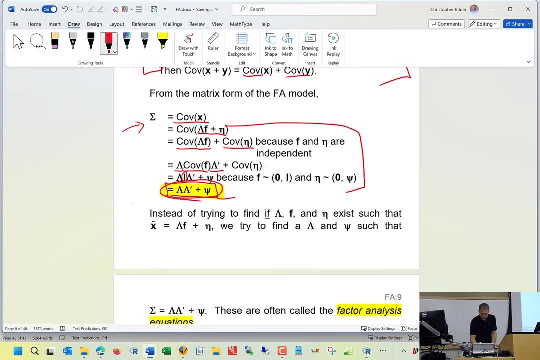 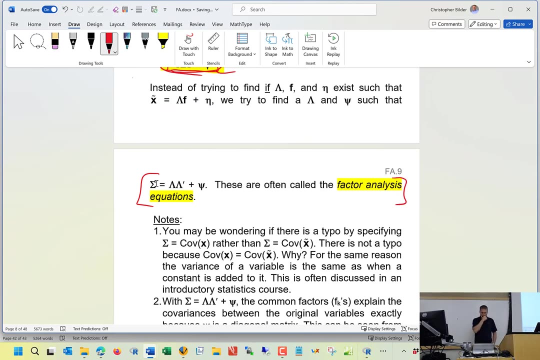 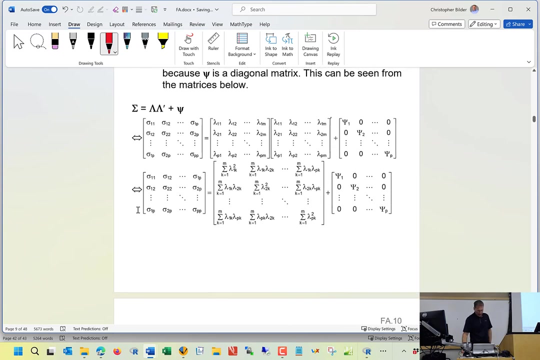 And so therefore, I'm left with this. Also, remember the covariance matrix of eta. we represent that symbolically by a sine, So that's where this expression comes from. These are: this is called factor analysis equation, Okay, And I think I actually added this to the notes. 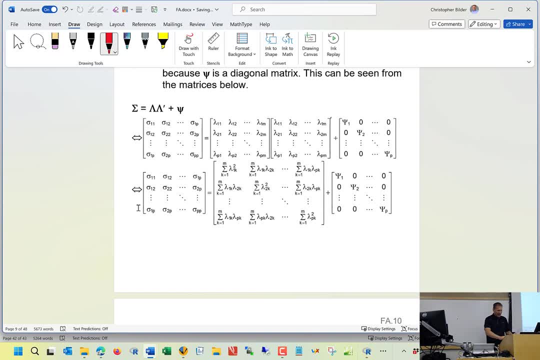 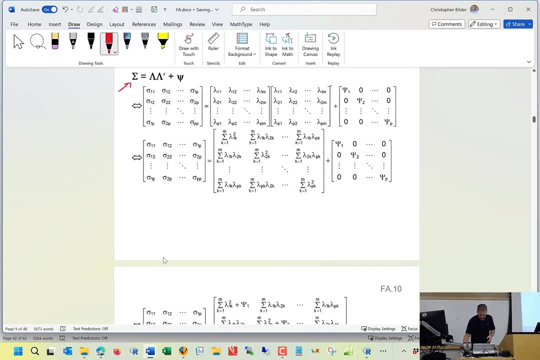 It's not that big of a deal because it's actually like two pages ahead. So you know what does this? what did I? No, I didn't, I didn't. This was there before, excuse me, So let's actually let me make this a little bigger. 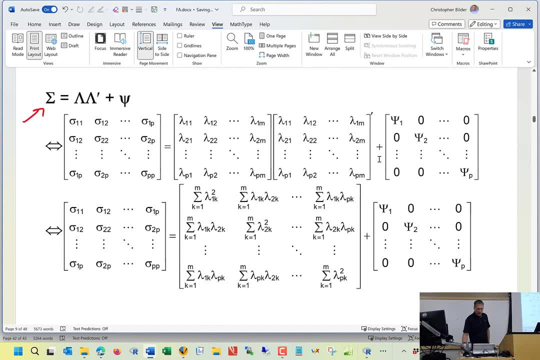 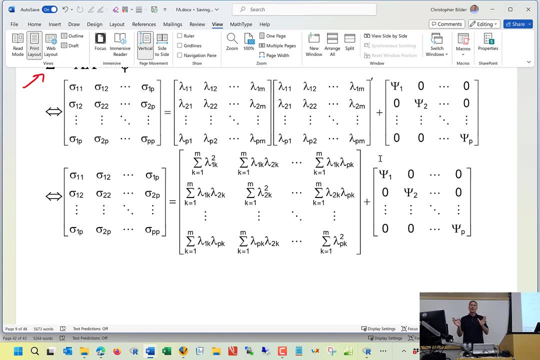 so we can see it better. You know it's often well. let me re-shoot that. Well, it's helpful to be able to write stuff in matrices. It's still often helpful to write out those common or each of the parts of the matrix. 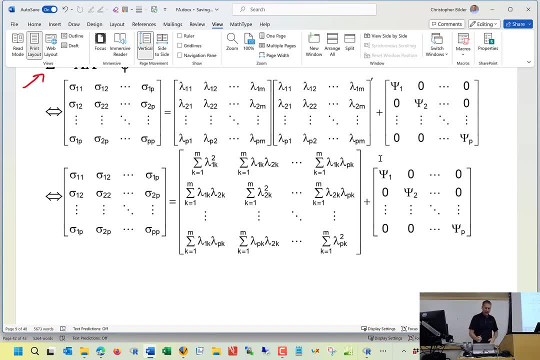 so you can better see what's actually inside of it, And so that's what I did here. So here's my covariance matrix sigma. Okay, So sigma one one would be, of course, the variance of x one. Sigma one, two, or little sigma one two. 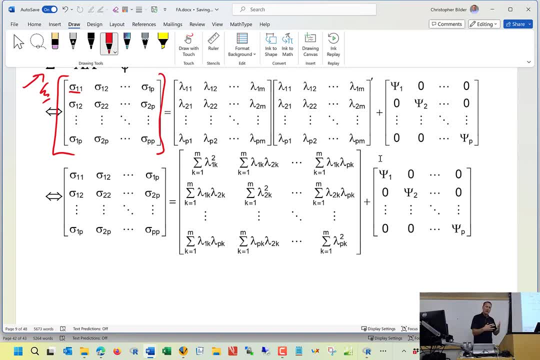 is a covariance of x one and x two, which represents the dependence between those two random variables. Then I have my matrix of factor loadings, Matrix of factor loadings transpose, plus then my sine matrix for the specific variances. Okay, Let's do some matrix multiplication. 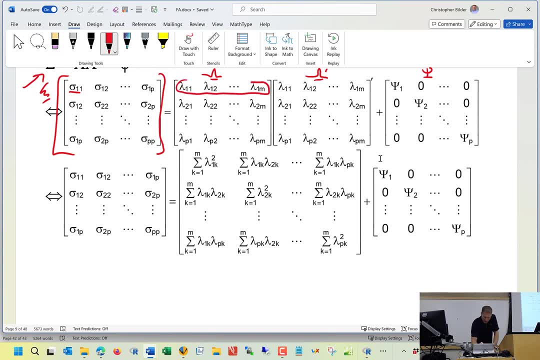 So, of course, what you need to do, you take the first row of your lambda and then you would multiply that essentially by that first column of your next row. So that's the first column of your next matrix. But remember what we have here. we have a transpose. 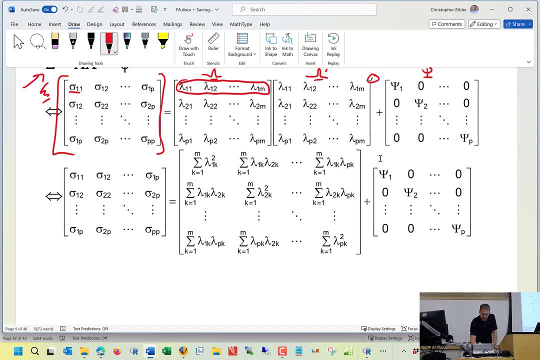 So I could actually write it out in terms of a transpose, and maybe I should have, But what that basically means is that now, after I take my transpose, this is gonna be my first column. So when I actually multiply those two out, look what happens. 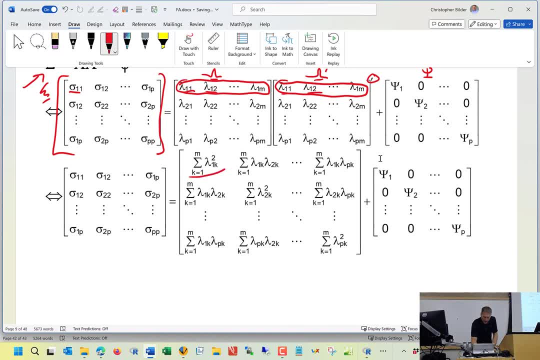 I have a lambda one, one lambda one, one, Lambda one two, lambda one, two, And so, in other words, I'm just squaring all the lambdas and I'm adding them up. Let's just do one more case. So let's let me. so that gives me my one, one element. 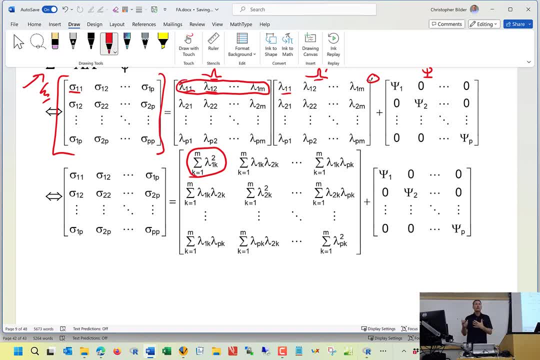 of lambda times, lambda prime, To get the one two element, I take the first row of lambda times. now what ends up being the second row of lambda because of that, transpose again And so look what happens then is I get. the sum of this is from that first row up here. 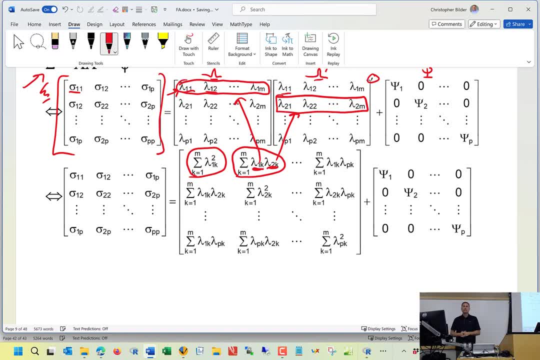 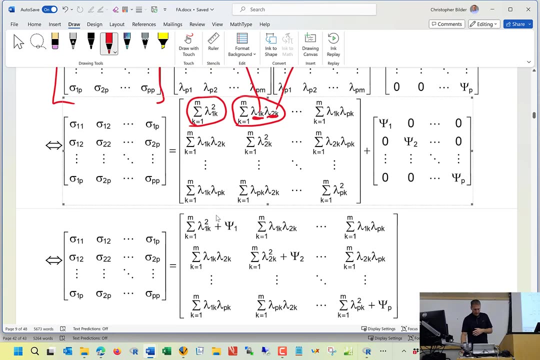 times that second, And so this. the end result is I have a bunch of these sums of the lambdas multiplied together. Next, How about we start moving, in the terms of my psi matrix, into this matrix of these lambdas that I just found? 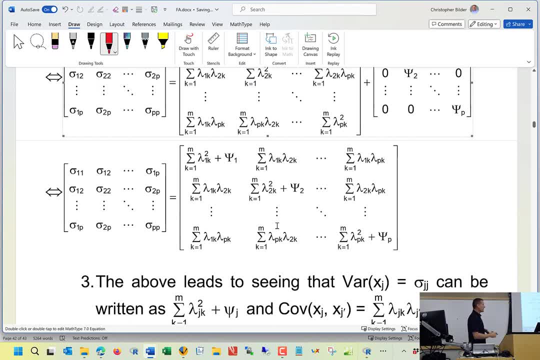 And this is what I end up with. You know, all the off-diagonal elements were zero for that psi matrix, so they don't affect anything, Just the diagonal elements. And so look what this means: Sigma one one is equal to, excuse me. 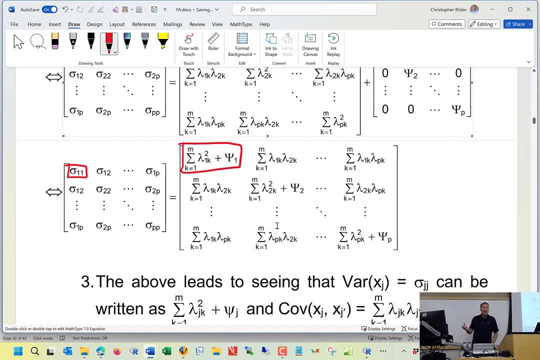 the sum of these lambda squared sigma one one is equal to excuse me. the sum of these lambda squared sigma one one is equal to sigma one one is equal to excuse me. the sum of these lambda squared sigma one one is equal to excuse me, the sum of these lambda squared. 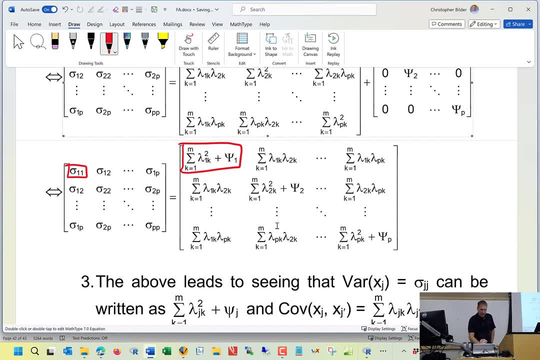 plus psi one. Sigma two- two has a similar representation as well. And then the covariances themselves, like little, sigma one two is equal to the sum of these lambda squared- I'm sorry, lambdas- multiplied by each other. Okay. 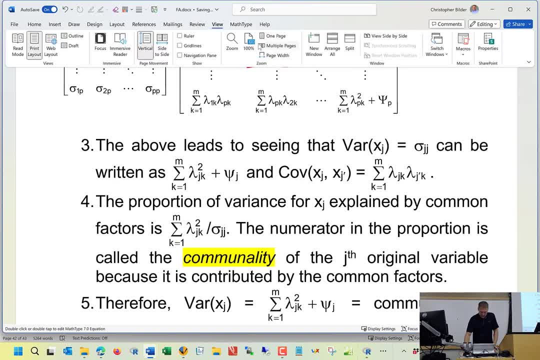 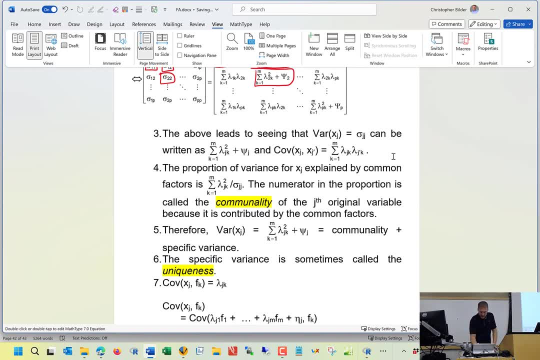 Let me make this smaller again. So, given this expression here- I guess I just kind of wrote this out- Each of the variances can be represented. variances of original variables can be represented like that. Now we have some more terminology. 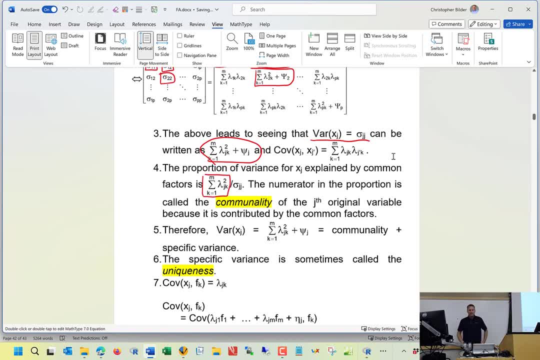 The sum of these lambda squares that's called the, what's called the communality. Why, Well, this is what's? these are the lambdas on F1, F2, all the way down to FM are common factors. 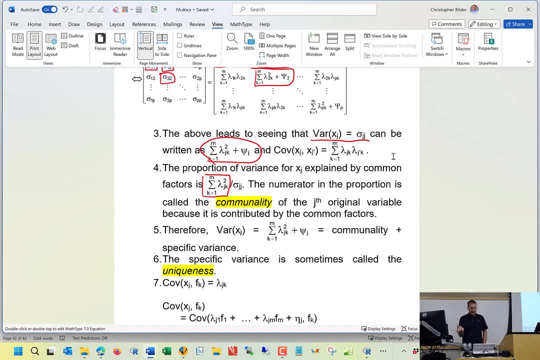 So that's where the terminology communality comes from, And we might be interested then, is well, what proportion of the variance of XJ is explained by the common factors? We just look at the sum of these lambda squared, That's it. 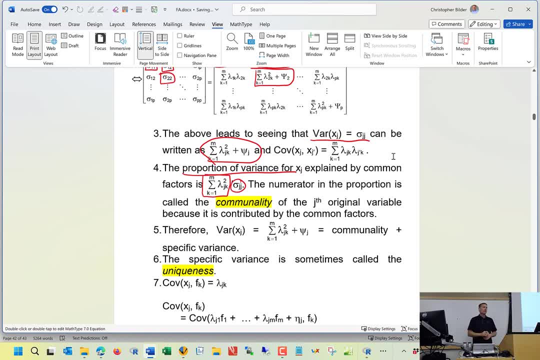 And for proportion. then we take the original variance for, let's say, X, J, And so you know- and perhaps this is overdoing it- The variance of XJ then is essentially equal to the what's called a communality plus the specific variable. 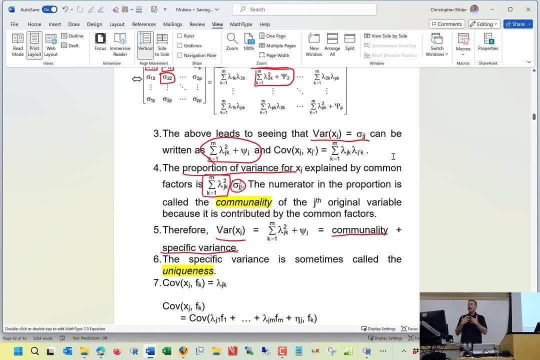 You can say: X matrix variance. Now again, if it was me, if I was the one who's inventing factor analysis and introducing these notations, I wouldn't even use the word communality. but I'm showing you this because others use it and you usually see this word in output. 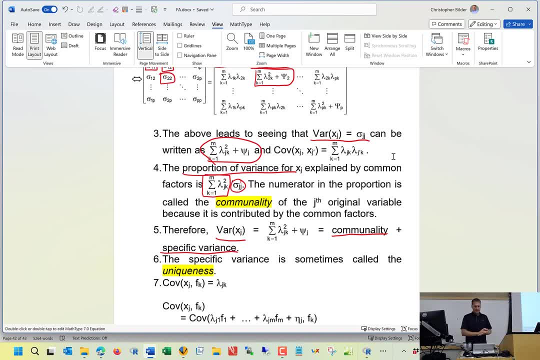 from R or even other statistical packages. Another example of this terminology: specific variances are often referred to as the uniqueness. Why? Well, you know, each of the specific factors are unique to a particular X, and so people often now refer to them, the corresponding specific variance, as the. 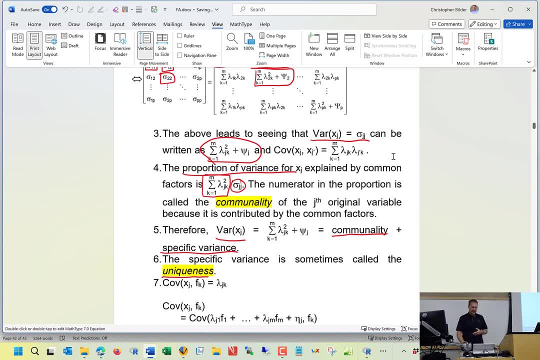 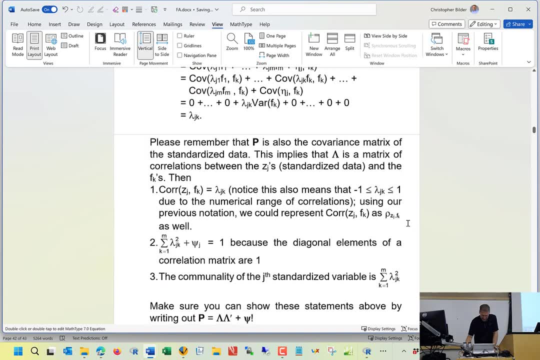 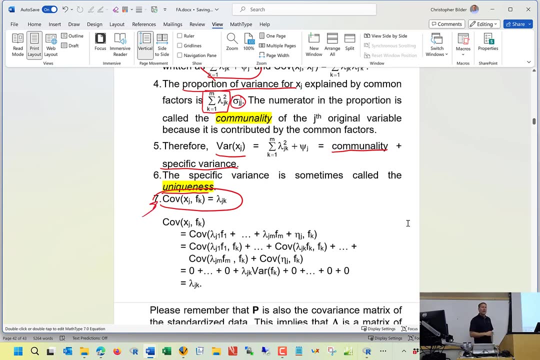 uniqueness. Again, you often see this in the output And let's see, I think we'll. we'll end it on this, Maybe not Okay Now. I said before that these lambdas are going to be very important to us. It helps us understand the 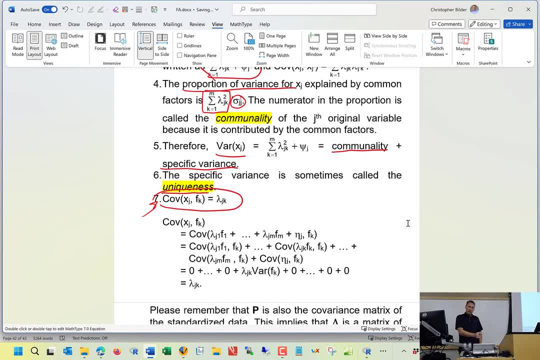 relationship between the common factors and the original variables. You know, we said if a lambda was zero on, let's say, F1, that says F1 plays no role into what, let's say, the corresponding X is. But we can even go a little bit. 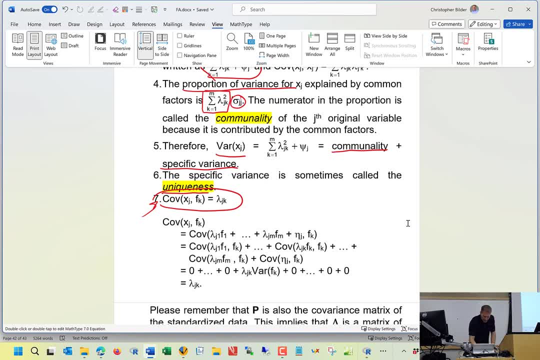 further, One can derive- and you are not responsible for the part that I'm circling right here, If you had a mathematical statistics course, one could actually derive that the covariance between XJ and FK, so one of the original variables, one of the common factors, 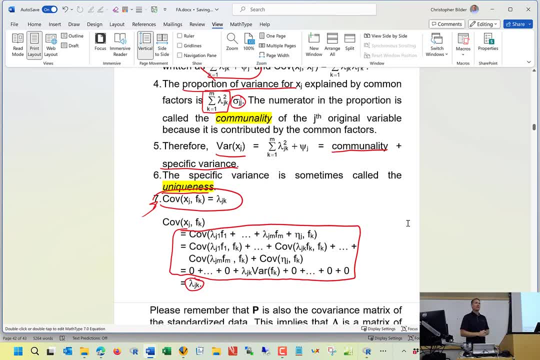 that covariance is lambda JK. So, again, covariance measures dependence between two random variables, And so now we have a nice little mathematical representation of just how important this lambda is, Because, again, if lambda JK was zero, that means that there's no association at all between the two. 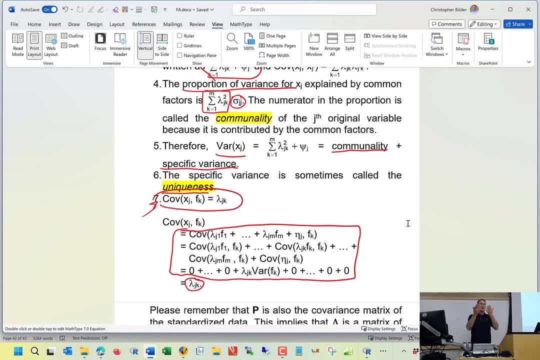 If lambda JK is, let's say, positive, away from zero, that says there's a positive dependence. If lambda JK is negative, that says there's negative dependence. And you can use that then to try to interpret what then the corresponding, what that corresponding? 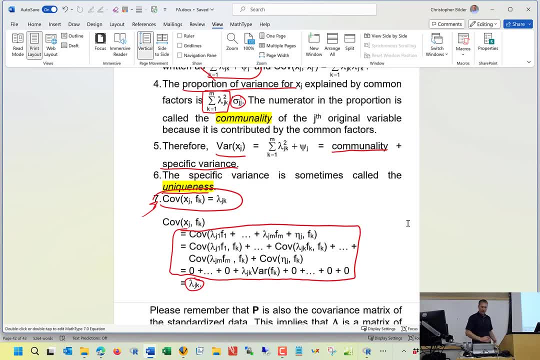 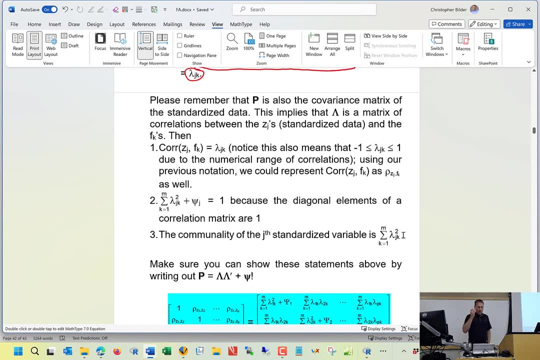 F is actually representing in terms of the original variables. We'll go a little bit farther here Now. remember, we will typically work with the correlation matrix, So that means then the correlation of ZJ and FK. then when we represent the model in terms of these, 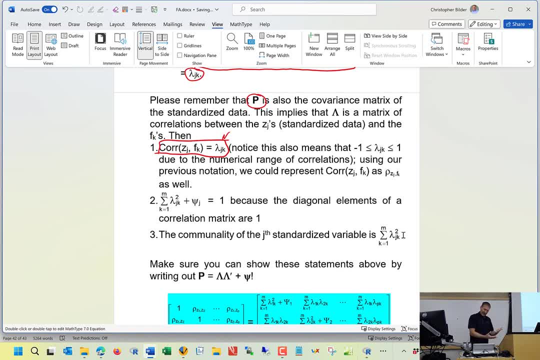 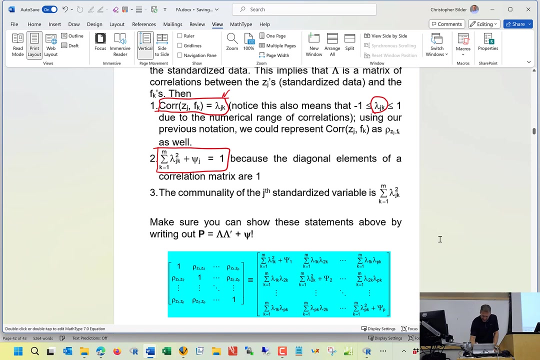 standardized variables. that correlation is lambda. JK Also remember each of those variances is essentially one Because we're working with standardized random variables. Also, these lambdas will have to be between negative one and one, because this is a correlation. 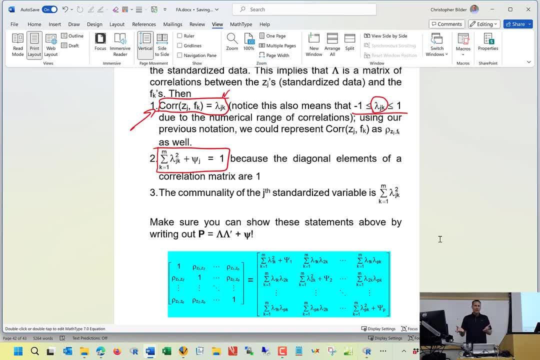 We will review this, obviously, next time, But there's a lot here And you know, one of my recommendations always, whenever I teach this to students, is actually write it out. You know, this is how we can represent the factor analysis model. 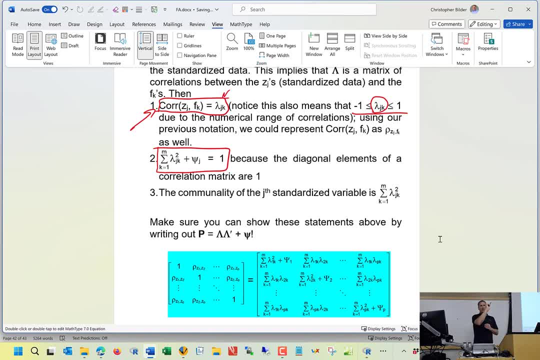 Here's another way. here's another way. This is the definition of communality. This is the definition of uniqueness. This is just write that out And almost think of it as like your study sheet. So this is the definition of commonality. This is the definition of uniqueness. This is just write that out and almost think of it as like your study sheet.